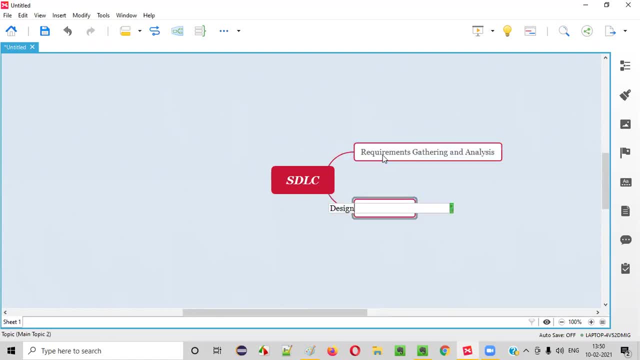 This is the first phase. Then the second phase we have is the design phase. Then we have implementation phase, which is nothing but the coding phase, you can say. Then, after implementation, we have the testing phase, then deployment phase And finally we have the maintenance maintenance phase. So these are the different phases of SDLC, guys. 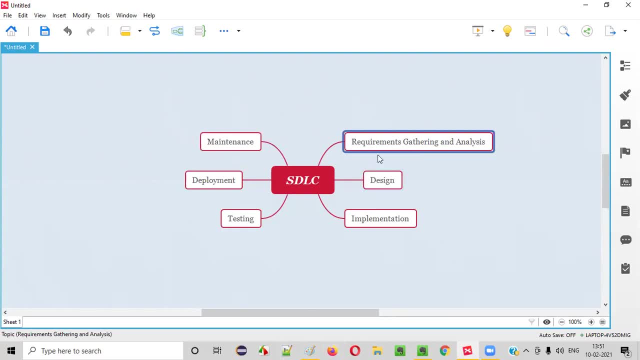 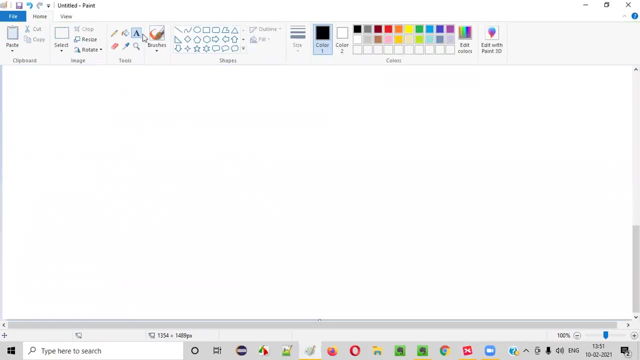 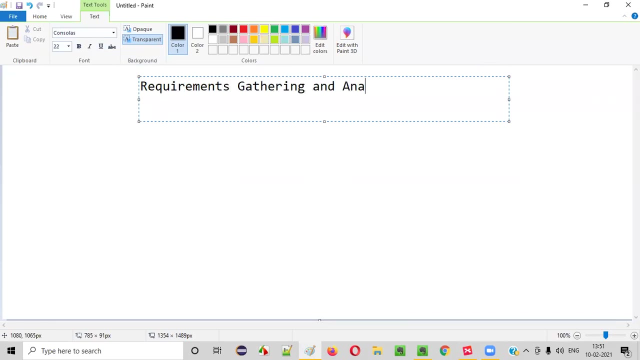 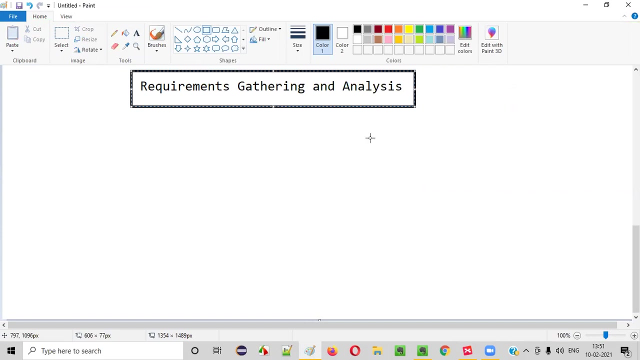 Now let me explain one by one. First, let's start with the requirements gathering and analysis phase. So first phase is requirements gathering and analysis phase. So first phase is requirements gathering and analysis phase. So let me start with scratch guys From scratch. let me start, Rather than directly giving you some definitions about requirement gathering and analysis. 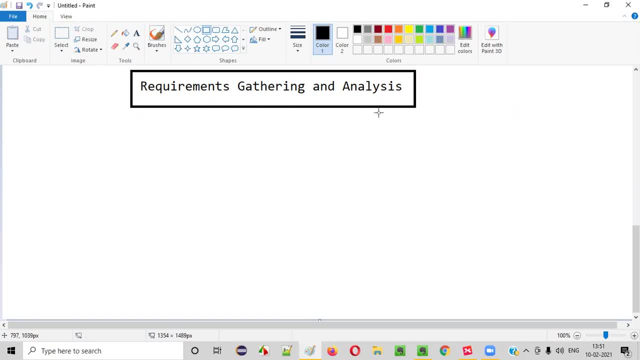 Let me give you some story kind of explanation so that you can understand this phase more. So it all starts with a person, guys, Let's say, let me name myself here, Let me give this person my name, Arun. Let's say there is a person say Arun. 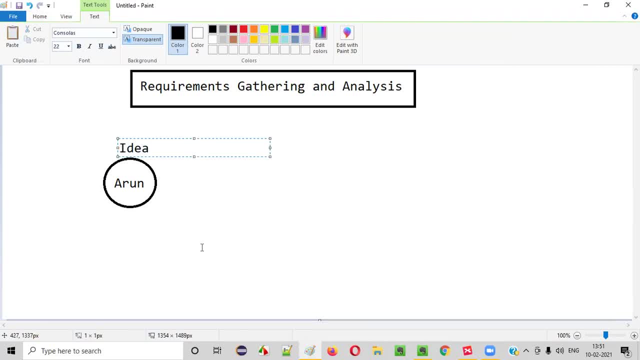 And someday he got an idea And he has some budget. also, This person has got some idea and he has some budget. And what is that idea, guys? The idea was to develop a software. The software is to like, let's say some random example: car wash, car washing software. 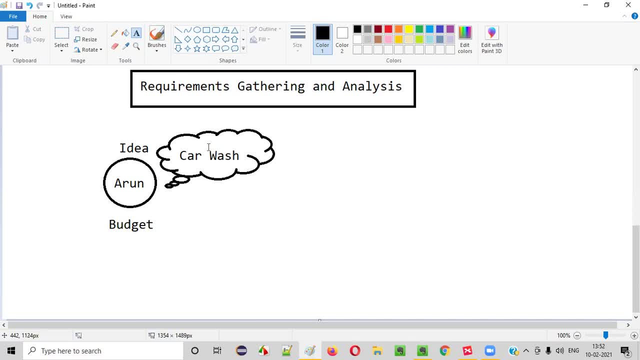 So where customers can book a slot for their car wash. So when they book a slot, a person from this company will come to the customer, collect their car, go there to the shed and then wash it and then return the car to the customer. 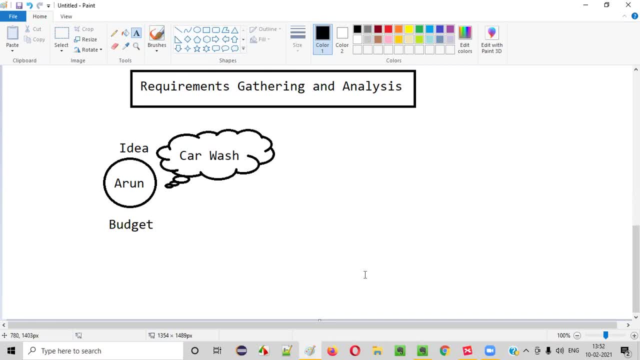 Let's say: that is what is the software at a high level. Let's assume: Okay, this is the idea this particular person, Arun, got, And he has a budget to make this software implemented and make it possible because he has the money. 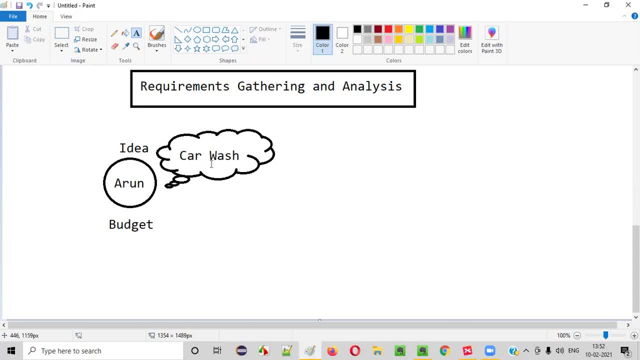 Now. but this person doesn't have much knowledge, guys. He only got the idea, but he don't know. He don't have any particular knowledge about this, cars and all the stuff. So what this person has done, He searched for another person. 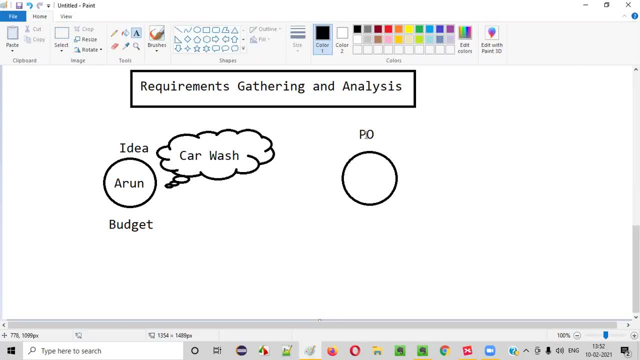 So whose role is PO? We generally call that as product owner. Okay, PO stands for product owner, kind of person he searched for. Let's say, this person's name is Kiran. Okay, this Kiran is a PO, product owner. 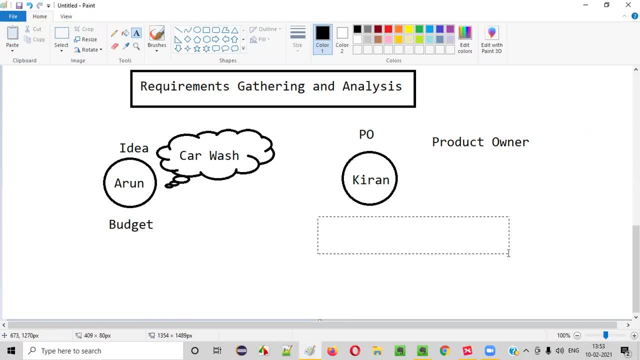 Why? Why Arun went to Kiran Because Kiran has good knowledge, guys, In this particular domain, in this particular domain of the software. this Kiran has very good knowledge. So Arun, who is, who has got the idea and has a budget to develop this kind of software. 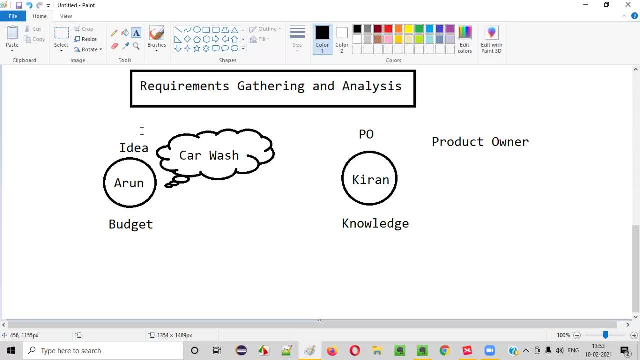 Since he doesn't have any knowledge, he went to this PO who has this knowledge about this area, And these two people will have meetings. Okay, so why Kiran will work for Arun guys? Why Kiran will work for Arun? 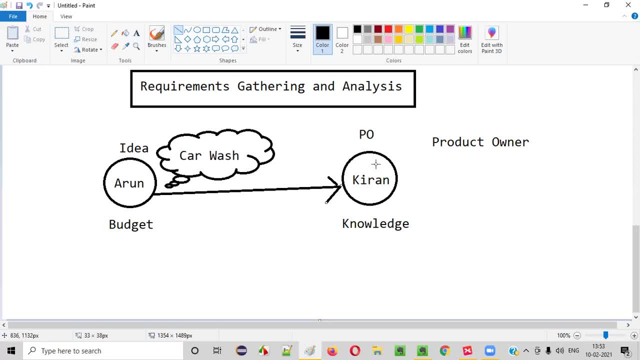 Because Arun is going to pay money to Kiran, right? So because he's having good knowledge. So Arun will pay money for his work, for his service as a product owner. Fine, Now, these people are good. Now, another thing is: when these two people meet, what happens is this: Arun will talk about idea, whereas Kiran will share the knowledge. 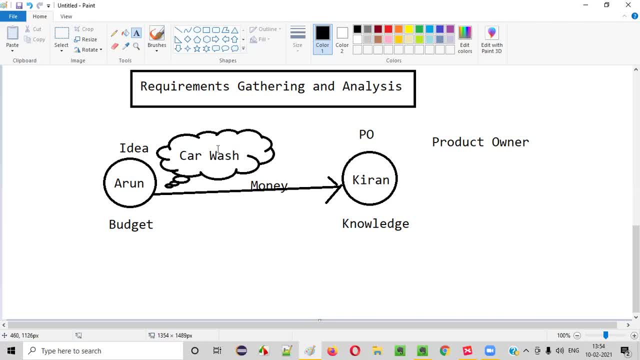 Like what we have to do for getting this particular software implemented. Okay, All these things, some discussions will happen. During the discussions we'll get a lot of requirements, guys. Okay, We generally derive During these discussions between the Arun and Kiran. that is, the one who thought of the idea and the one who is called as a product owner here. 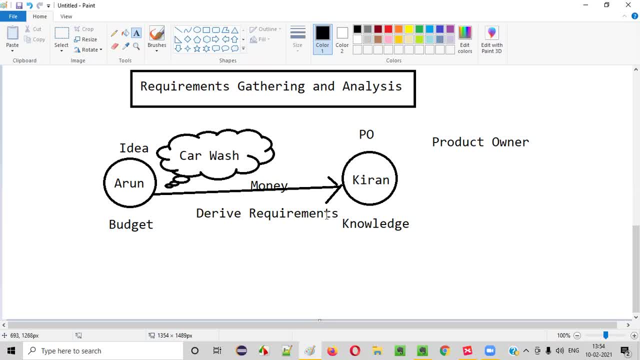 During their meetings. they will get a lot of requirements. guys, A lot of discussions will happen out of the discussion. This will work, this will not work, such kind of discussions- Then a lot of requirements can be derived. So for writing this requirements in a proper way. 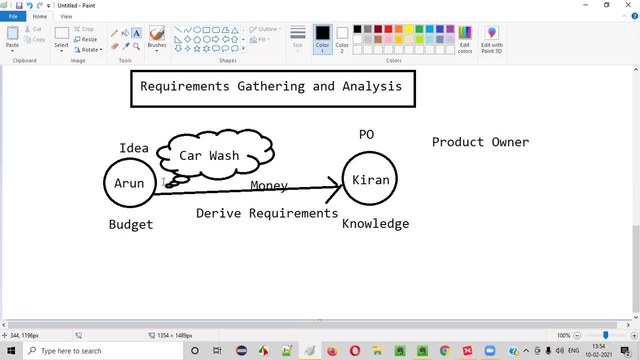 Okay For making this requirements thing gathered in a proper way. what this Arun and Kiran will do is they will appoint one more person. Generally we call that person as BA guys. Okay, BA, Let's say this. BA is Praveen. 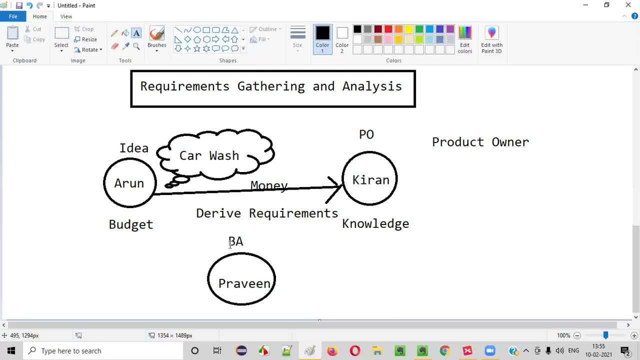 His name is Praveen Okay, Business analyst. His role is to. His role is to attend these meetings between this Arun and Kiran- That is the idea created- and the product owner as a BA, and understand their conversations and derive the requirements. 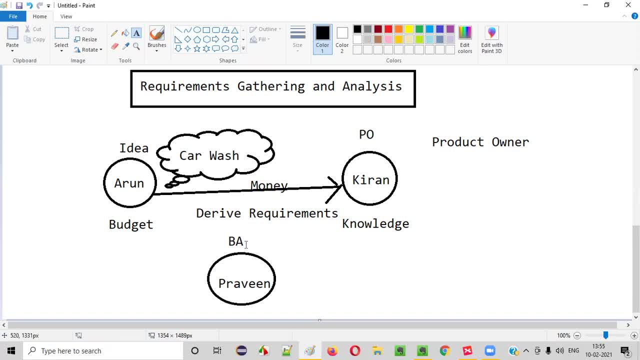 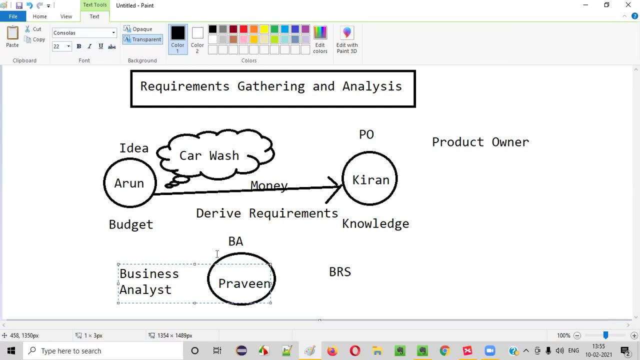 This BA is very good at gathering the requirements and creating some kind of documents like BRS document. So BA is a person. Business analyst, BA is nothing but business analyst guys. Business analyst- This person is responsible for creating this BRS document, guys. 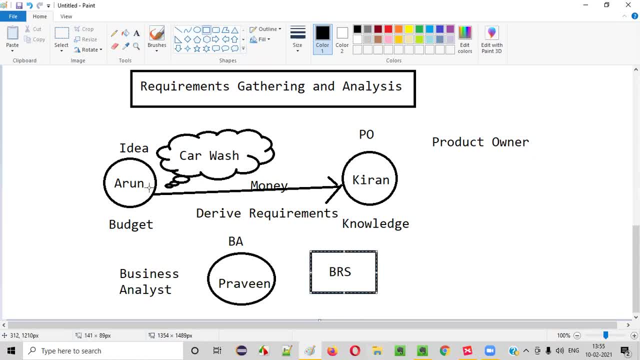 Okay, So he will attend these meetings with the Generally this: this person who came, who got the idea and who got the budget right, He generally will be called as client in the later time. Okay, Later time, Once this project starts right. 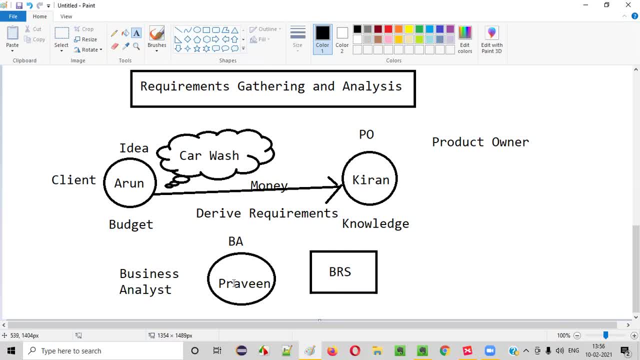 This person will be called as client And this one is product owner And this one is a business analyst Who is bothered about communication part. Okay, He is bothered about communicating the requirements. guys, Business analyst is all about communicating the requirements. Fine. 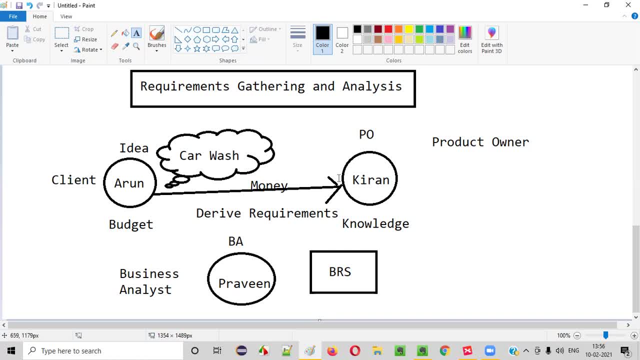 So BA will be there at the client side starting from the beginning When this discussion starts with the product owner and the client. BA will be there in this meeting and he knows everything from beginning And he creates this BRS document. Okay, 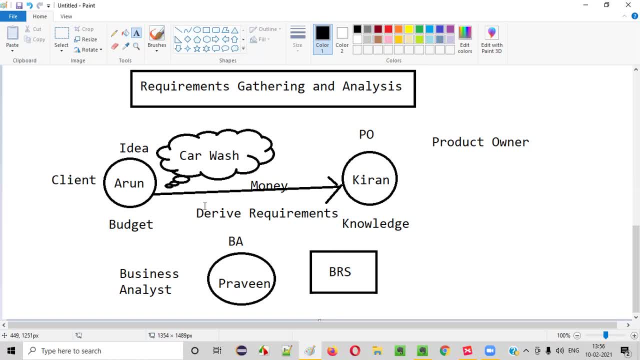 Once this discussions are finalized, Once this discussions between the client and product owner are finalized in several meetings, This BA will come up with this kind of finalized version of the BRS document. guys, Fine. So this phase, This phase where this kind of situations are going on between the client, product owner, 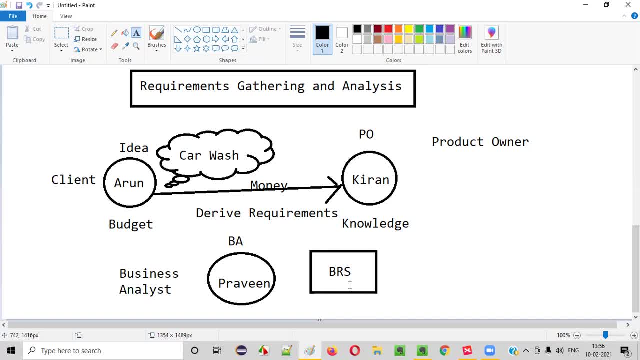 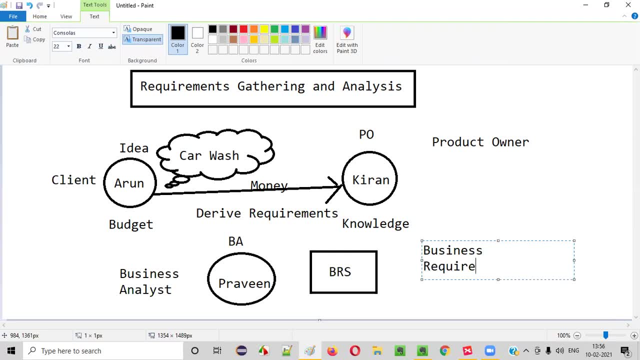 and business analyst where the output is this BRS document, business requirement specification document. What is BRS- Business requirements specifications document? So the output of this This phase is requirements phase guys. Okay, Whatever the phase, I am explaining right. 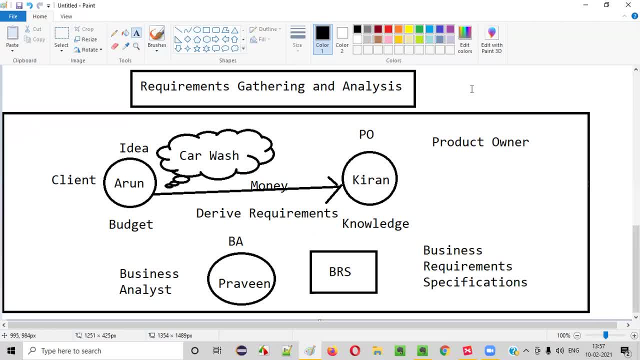 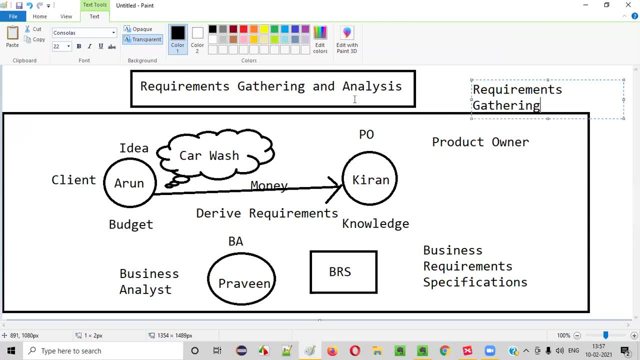 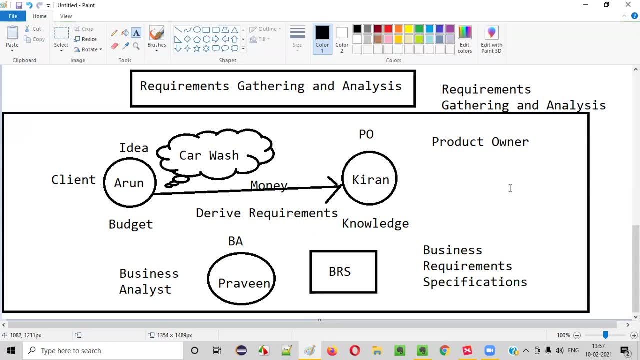 Whatever is happening, This is happening. in which phase, guys? Requirements gathering phase. Okay, Requirements gathering phase and analysis phase. you can say, Okay, Requirements gathering and analysis phase. This particular things are happening, guys. Okay, The output of this particular first phase is BRS document, which is created by this BA. 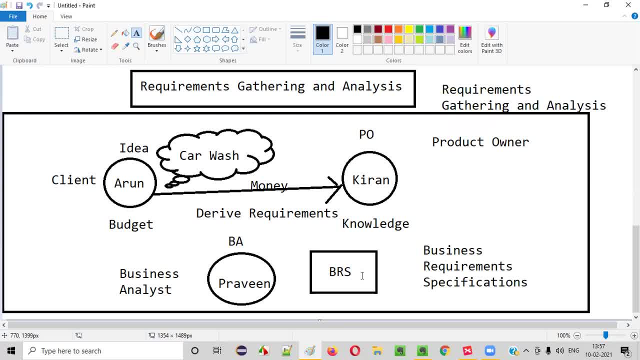 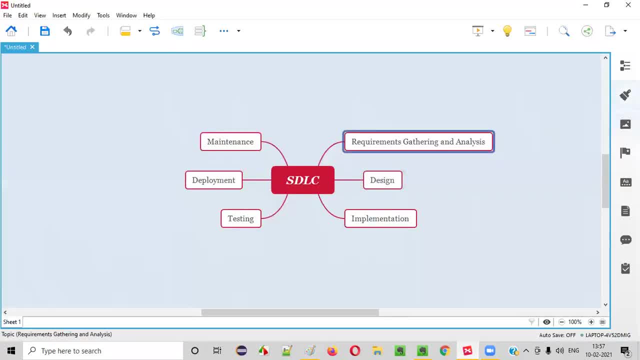 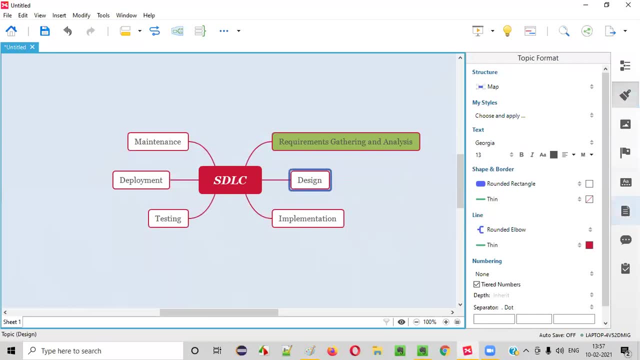 Drafted or created by this BA. Okay, This is BA business analyst, which is fully called as BRS, fully called as business requirements specifications. So hope, guys, you understood what exactly is this: requirements gathering and analysis phase now. Now let's move to the next phase. 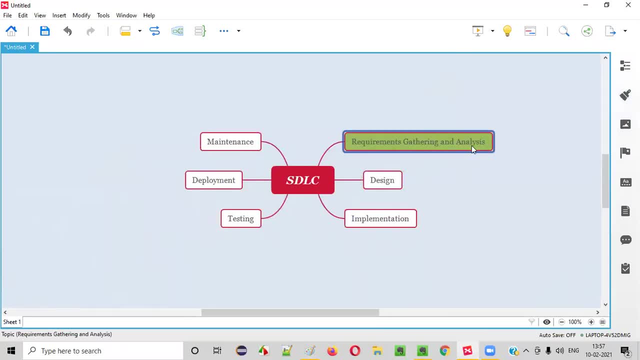 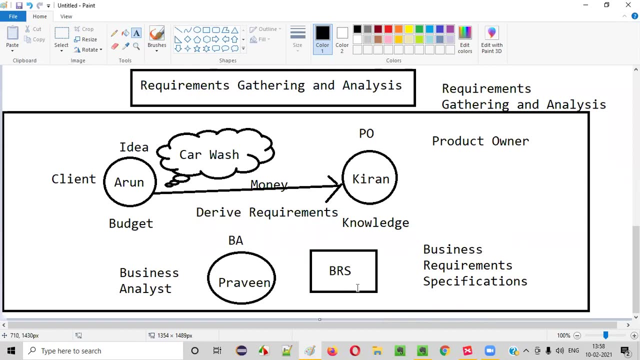 So before moving to the next phase, guys, there's one more thing with this requirements gathering and analysis phase. So later what happens is later. what happens is now: BA has created this BRS, all the discussions are done between the client and the product owner, and BA also has created this, finalized. 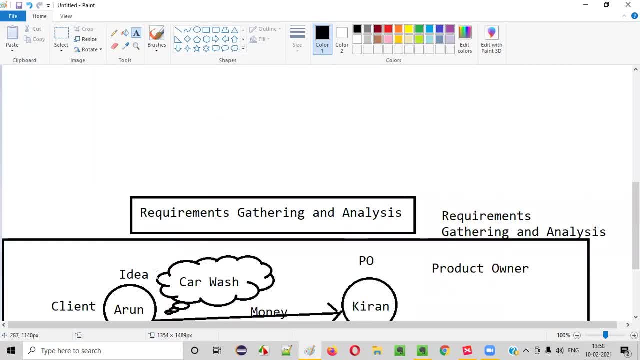 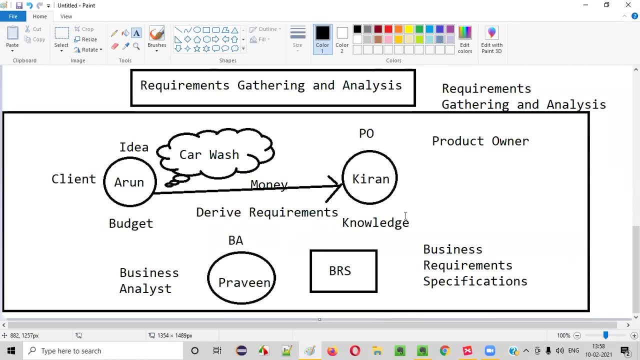 BRS document. Let's say, fine, Now, tomorrow, what this client will think is he want to hire or outsource this development work of this particular software. Okay, Whatever the BRS requirements are gathered for the software right That work, he want to outsource this to another company. 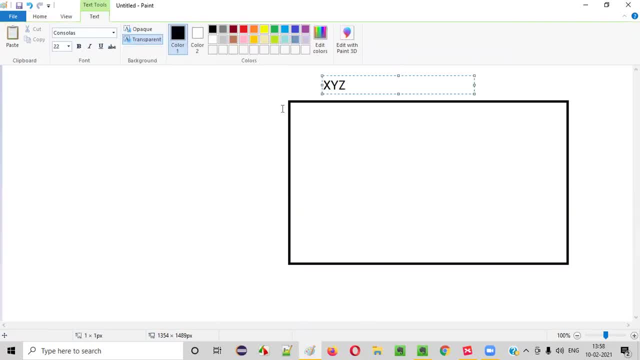 Let's say there's some XYZ company. This XYZ company has a lot of team. Big team is there, Like some developers are there in this, in this company, some testers are there, Okay So, and a UI, UI, UI people, a lot of people are there as UI, UX and all those stuff. let's 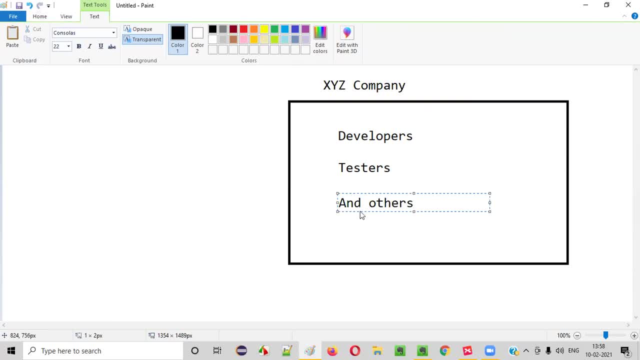 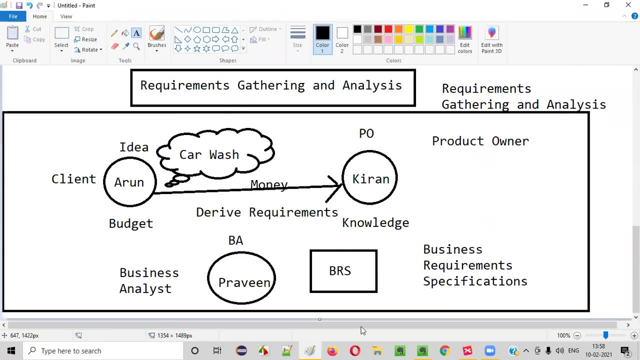 say Okay, And others. I will say simply, I will say others and others. generally, the major ones are developers and testers, right, And there are many other roles also, And there are many other roles also in this company And this, this development work, is outsourced by this client. 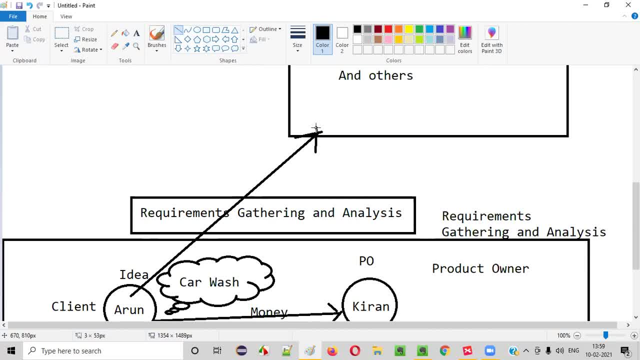 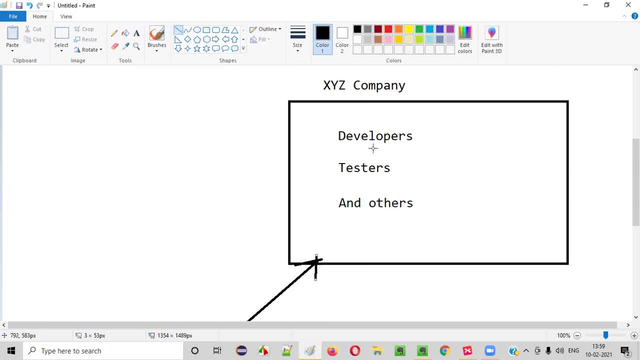 Let's say, the client has outsourced this development work to this company, XYZ company, Where we have this developers and testers in place. Now, now, guys, what this? uh, first, initially, it will all start with the development team. There's okay. 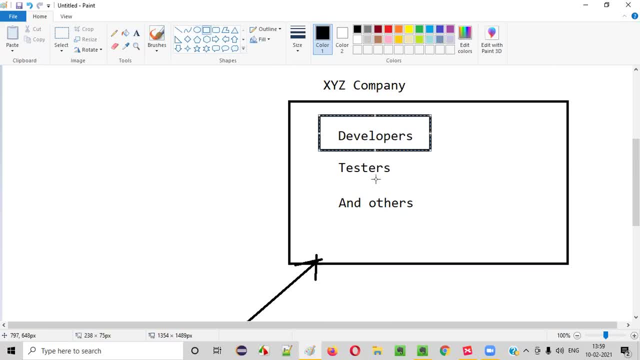 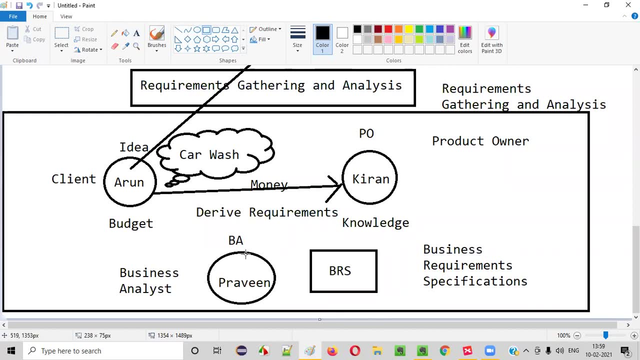 Testers may or may not. Okay, Testers may come a bit late compared to the developers. a bit early developers will be Okay. So here this business unlist. that is Praveen. Okay, We'll share this BRS document. 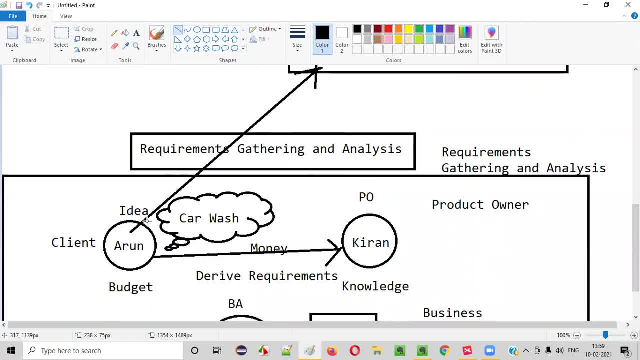 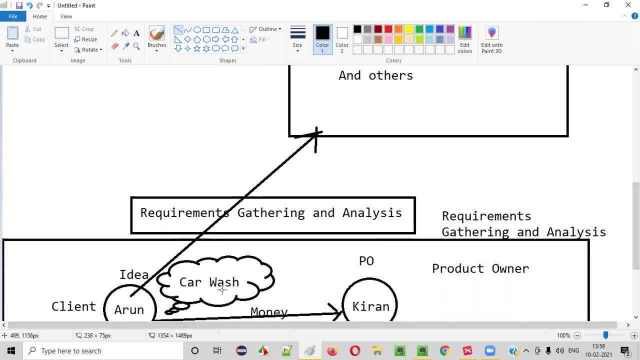 This Praveen is. So once this client has outsourced the development work to this XYZ company, Then the project starts here. guys, Okay, For this XYZ company. This particular development project will start here for this XYZ company, the car wash project. 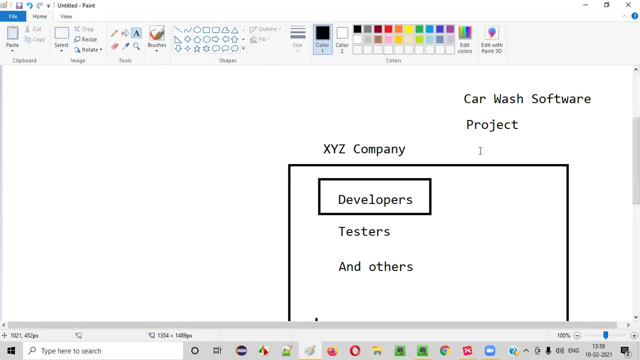 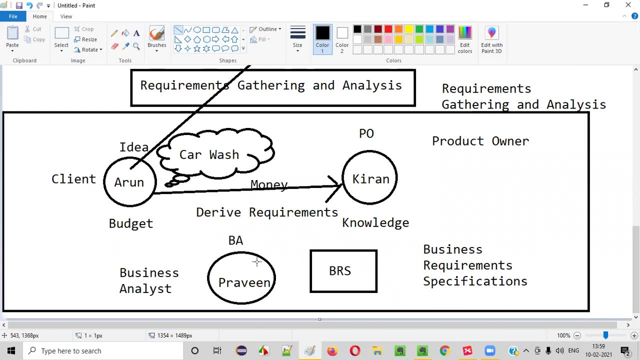 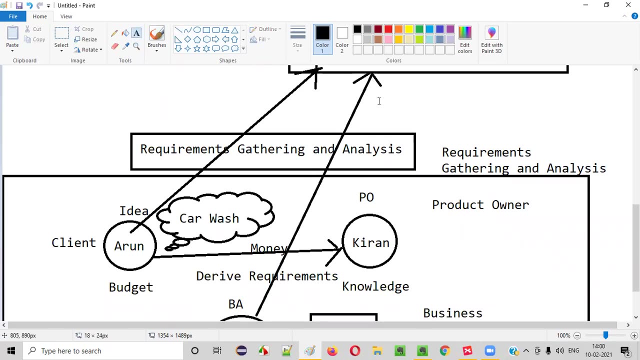 car wash software project starts, development project starts. Once this project starts, as a first step, this Praveen, who is a business analyst, will share. Okay, This Praveen will share the BRS document with home guys, with the development team first. 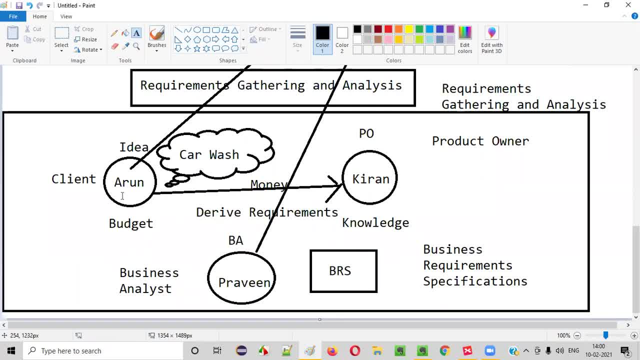 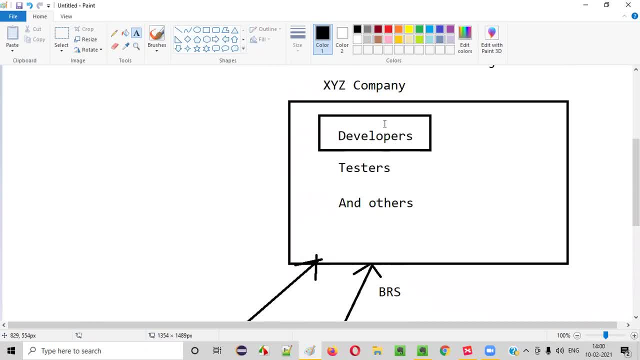 Okay, BRS document- business requirements specification document. All the discussions done by the client and the product owner will be drafted properly in this BRS document. that BRS document will be shared with the developers- developers- what they will do. Developers will go through this BRS document and see the possibilities. 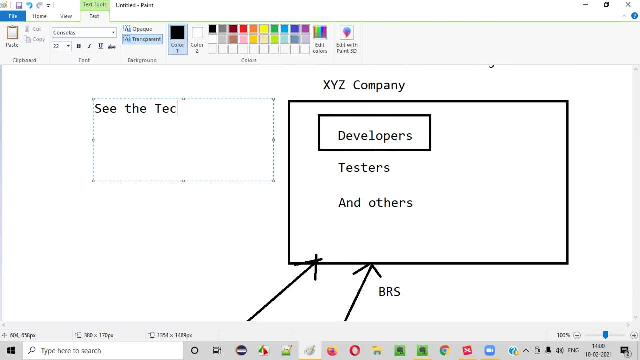 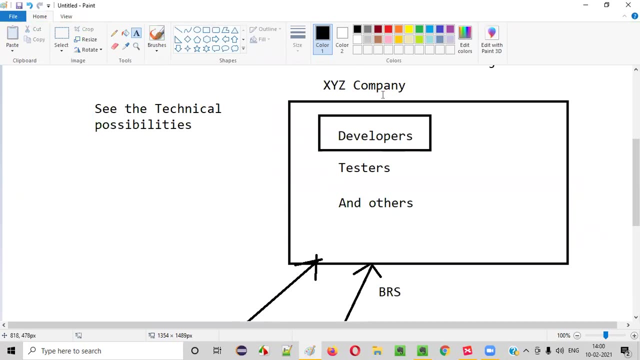 Okay, Developers will see the technical possibilities- You can say technical possibilities Of developing projects. Okay, Okay, this application. okay, what are all required at a high level? they will have some meeting or discussions. guys, development team of this xyz company will go through the requirements and see. 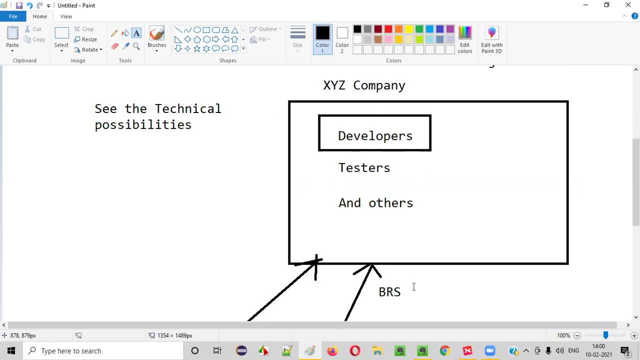 what is the best way of doing this, which technology we have to use, okay, what we can do, any other technical problems we get in future, or not? okay, so is it possible to even develop such kind of software using the all the tools and technologies we have and the skill set we have, all these things? 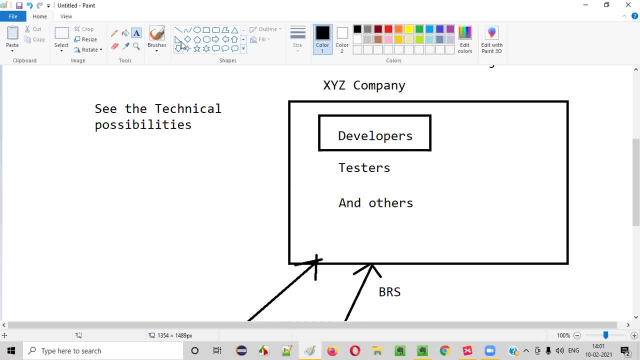 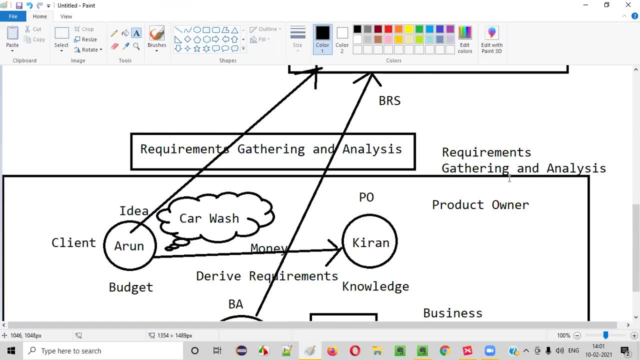 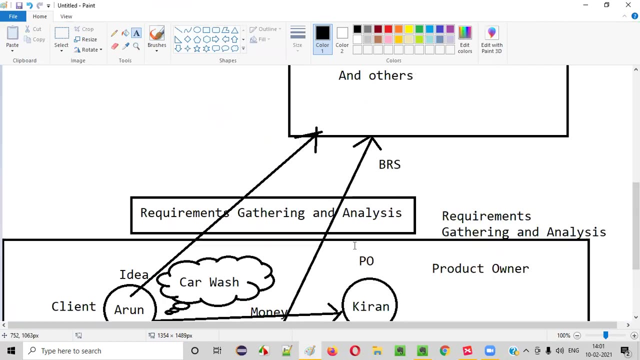 they will discuss, guys, okay, and they will come up with some document, guys, after this discussion. that means some analysis is being done by these developers. guys, in this requirements gathering and analysis phase, requirements gathering are done by this client, product owner and ba in form of brs document now coming to the development team of the xyz company. they will do analysis, technical. 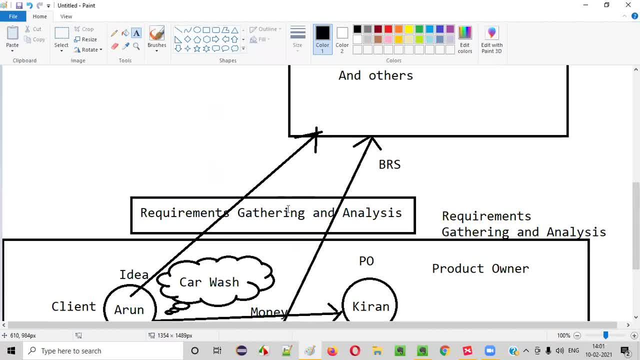 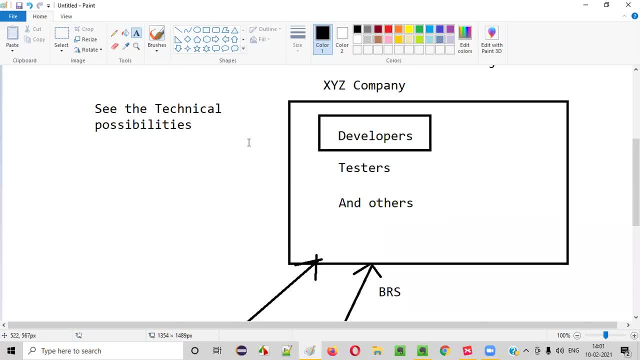 analysis to see whether, what are the technical challenges, which tools we have to use, technical tools we have to use, which programming language we have to use, which tools we have to use, which to use. such kind of discussions will go and see if it is possible to technically develop such kind. 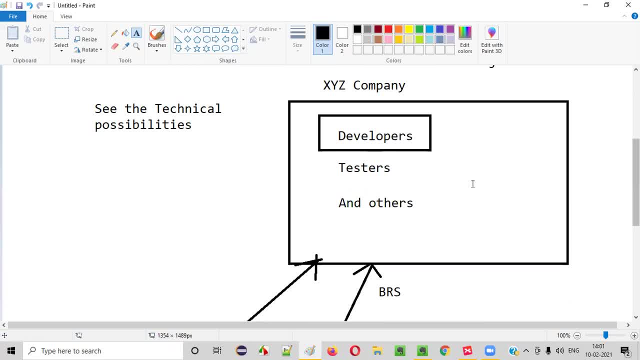 of software if we uh, in the coming days such kind of thing. so based on their understanding guys, they will create a document, technical document. so as software testers we don't have to bother about this. what this particular srs document will have, okay, so at a high level it will have the technical. 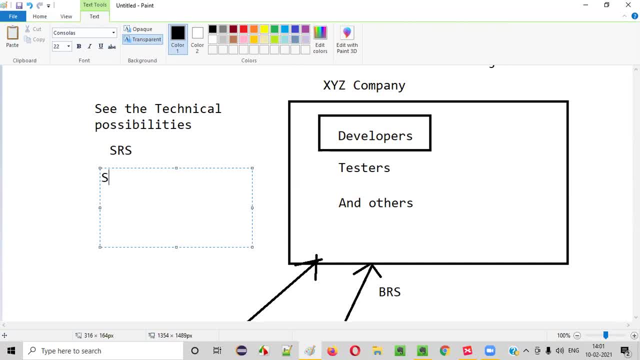 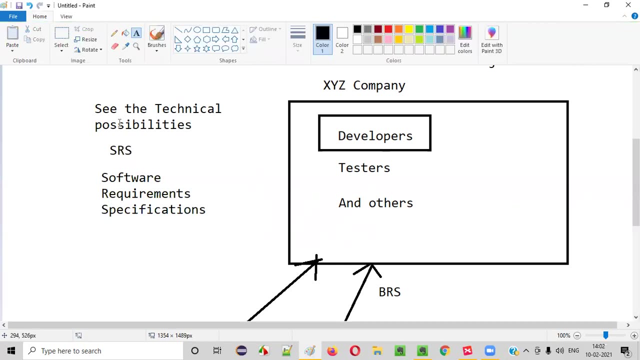 possibilities and what tools they have to use, and all the stuff. okay, software requirement. this srs is nothing but software requirements, specifications for the requirements. what are the software specifications required? okay, so that will be provided in this srs document. technical specifications will be there in this document, guys, and this document will be shared by the developers. 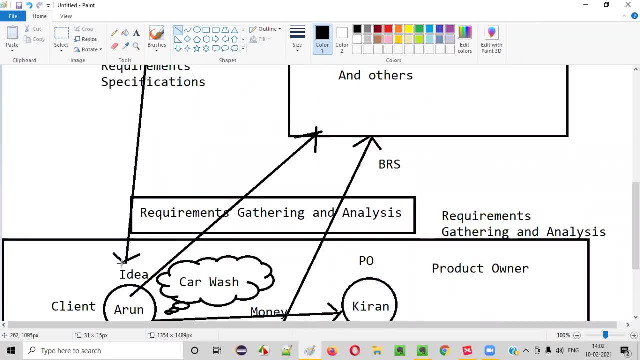 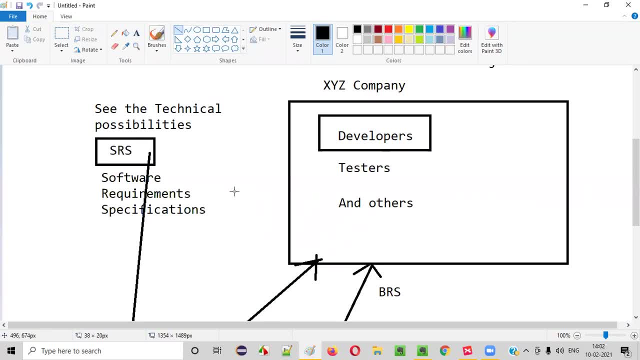 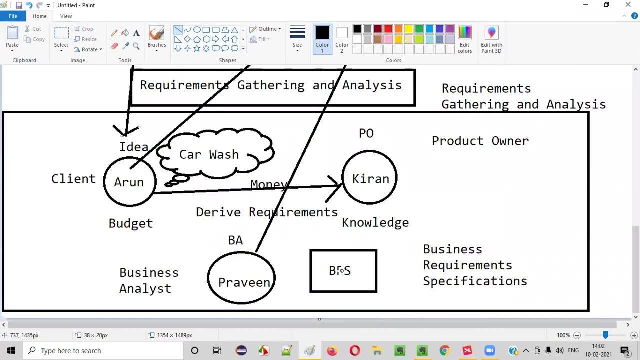 with the client. okay, they will be sharing this uh kind of document with the client once the client approves this, once the client approves this srs document, okay, and even during this process, guys, developers may also clarify few things about this brs. if developers don't understand few things about brs, right, some business requirement specifications if they don't. 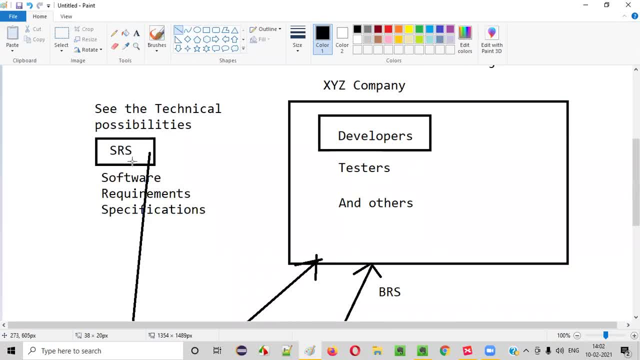 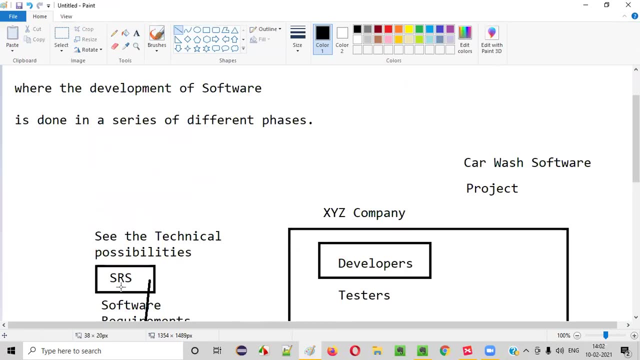 understand, they will simply ask the client team and get it clarified and finally, they will come up with the srs document. based on the technical possibilities of developing the software, they'll come up with a srs document. so this phase in which this brs and srs is coming out from the client side. 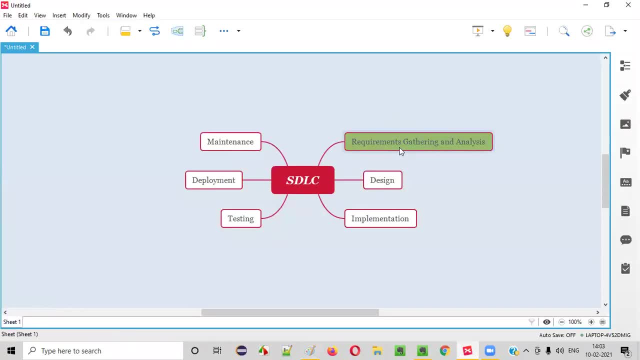 of the development team of this xyz company. that phase is known as requirements gathering and analysis phase, guys, so hope you got some idea. what is this requirements gathering and analysis phase? now let's move to the next phase, guys of this sdlc, after requirements gathering and analysis. 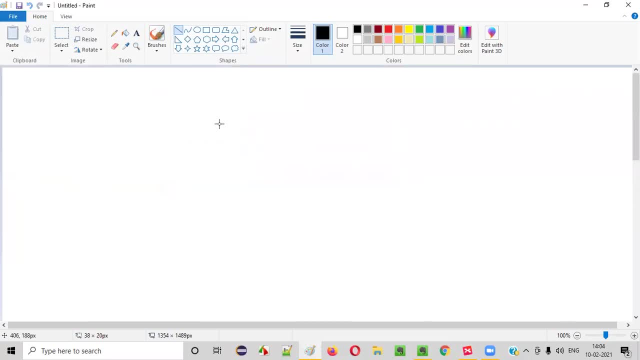 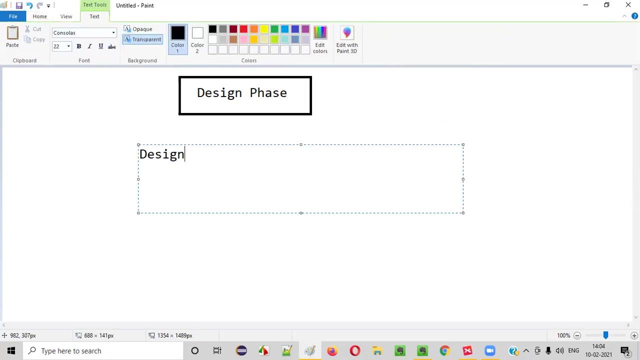 we have the design phase. let me explain the design phase now. in design phase: okay, the second phase in sdlc is design phase. in design phase, what will happen is the design team first of all, the team will create a design plan. okay, in design phase, the development team will create a design plan. 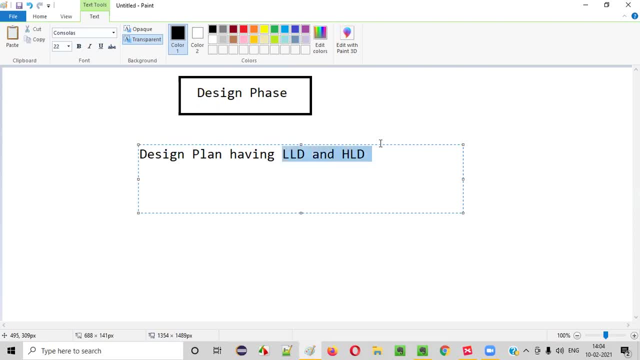 having low level designs and high level designs, lld and hld, low level design and high level designs. so low level designs can be as simple as the ui screens and all those stuff, and high level designs are, like you know, the architecture of the application to improve the performance. such kind of things, guys. okay, very technical. you can say. 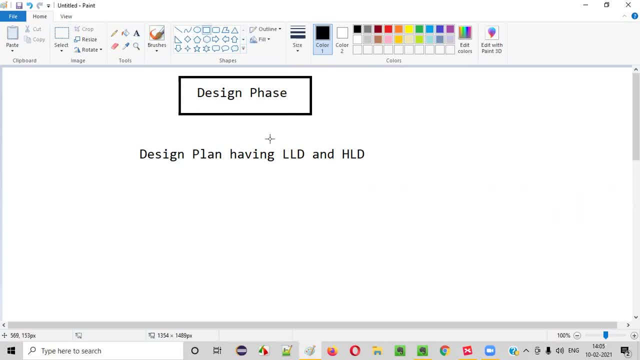 as software testers, we may not have to know what exactly is this: lld and hdl, hld. okay, lld and hld, so a technical plan, you can say technical design plan, for implementing the, for developing the software, like in order to develop this software in the coming phases. what is a plan? what is a 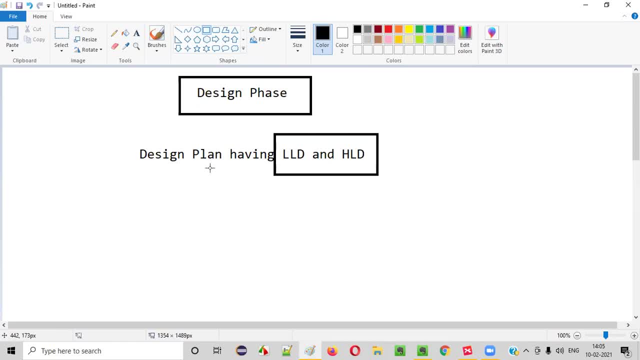 technical plan. they are going to create this plan. for this plan, guys, they are going to use this srs document. the previous phase development team has created this srs document. right, technical documentation was there about the application possibilities and all the stuff, tools and all based on this srs plan. they will derive this design plan according to this srs whatever. 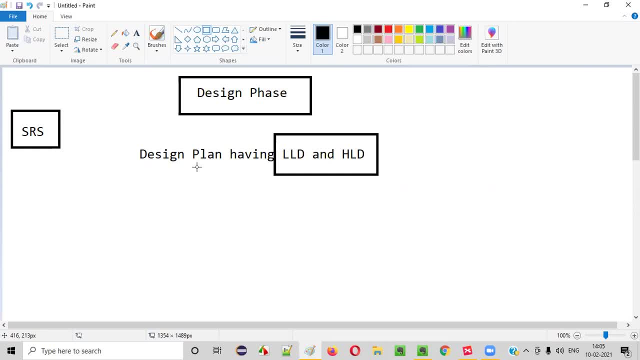 that is provided in the srs. they will create a plan guys. it's a kind of development plan. you can say they will plan their development in terms of this lld and hld. so low level designs and high level designs that are all required for developing the software will be created by the. 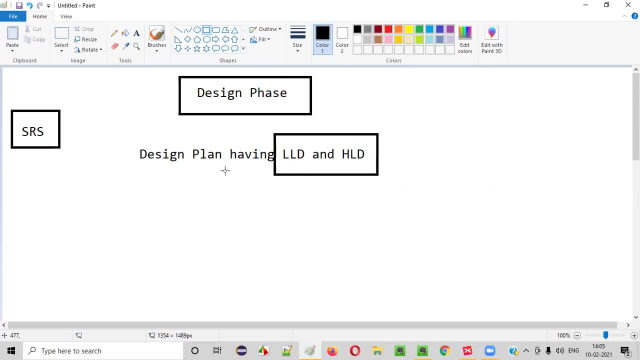 srs document. the previous phase development team has created this srs document. right technical development team, the design phase development team, will create this design plan based on this srs and and the output will be lld and hld. guys, okay, low level designs and high level designs, all the. 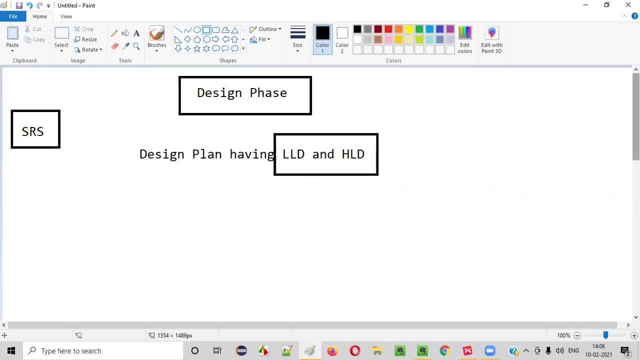 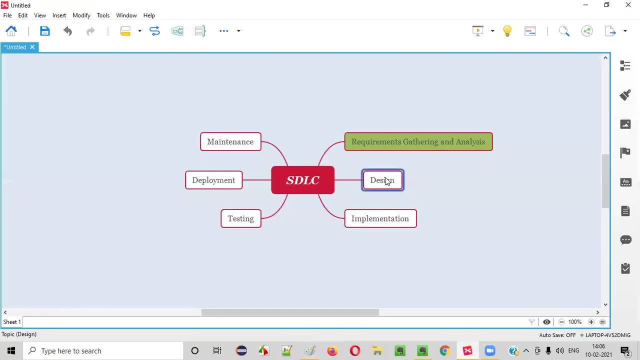 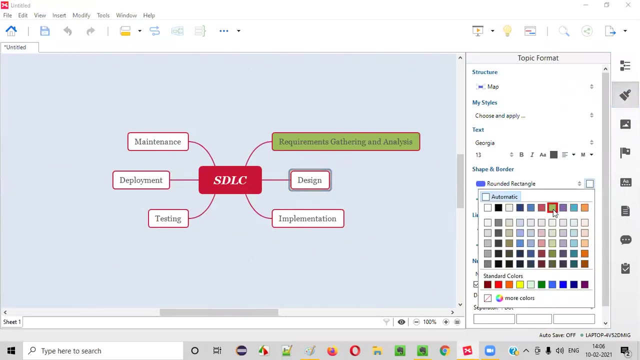 designs: architecture level designs, ui level designs- okay, they are very technical, guys, you don't have to understand that much. so once the design phase is done, guys, okay, once the design phase is done, then we are going to move to the next phase, that is, implementation phase. so once this srs document is approved in the requirement gathering and analysis. 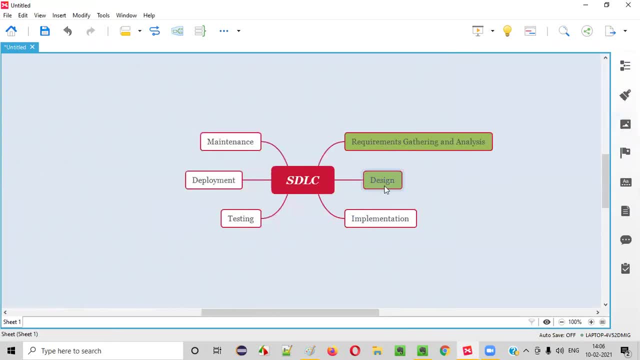 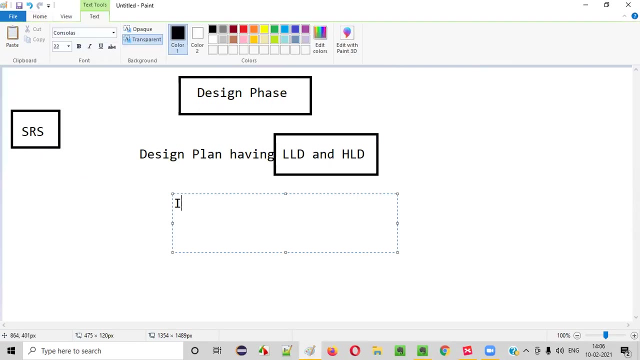 phase and the this design plan that is created by the developers- low level designs and high level designs, okay- created by the developers in the design phase- is also approved, then developers will move to the next phase. that is, next phase is implementation phase. the next phase is implementation phase. implementation phase is nothing but the development phase, guys, okay. 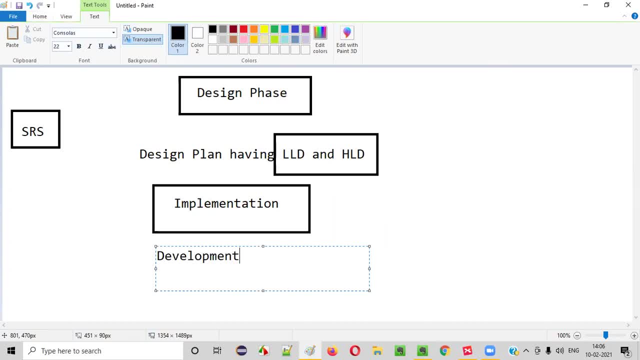 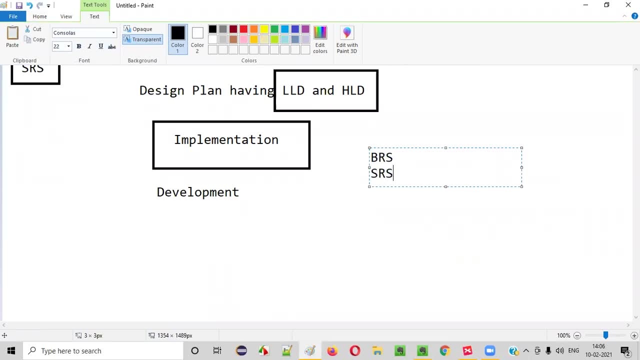 implementation phase is nothing but the development phase. according to this brs. okay, according to the brs business requirement specification- uh, software requirement specifications and this design plan, which are created as part of the previous phases. development team will start writing the code. okay, the development team will start. 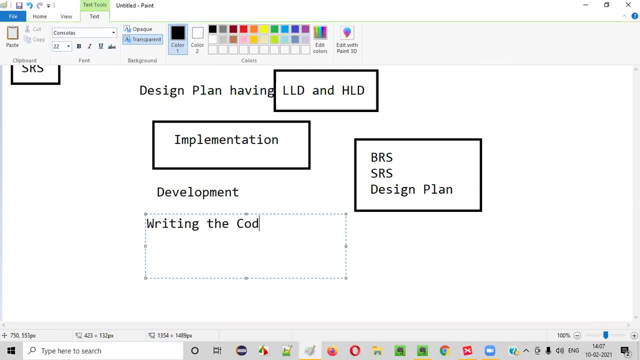 writing the code. that is, they do the actual development. they will write the code in order to develop the software. that developing the code will happen. in which phase? guys? implementation phase, developers will develop the software by writing the actual code for developing the software in the implementation phase. 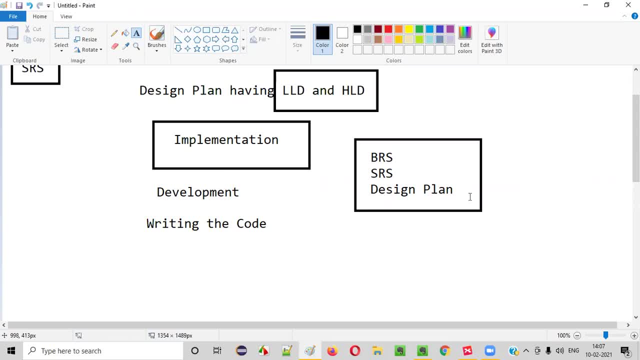 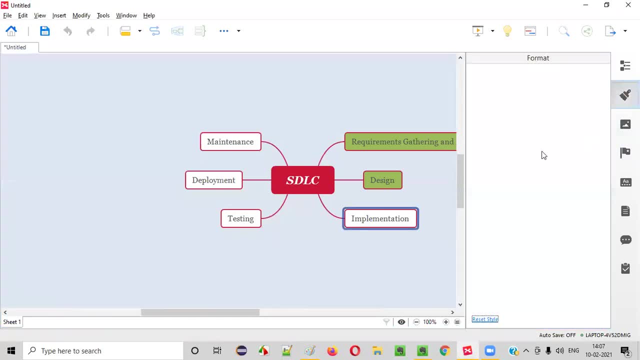 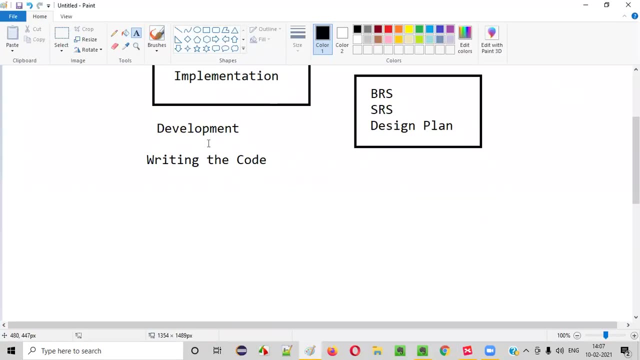 For writing this code. they follow this BRS, SRS and design plans. Fine Done. Next one: after implementation. After implementation, the next phase we have is a testing phase. Let's say the developers have written the code, completed writing the code for. 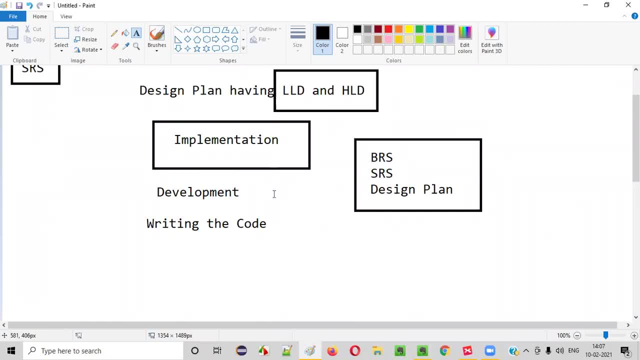 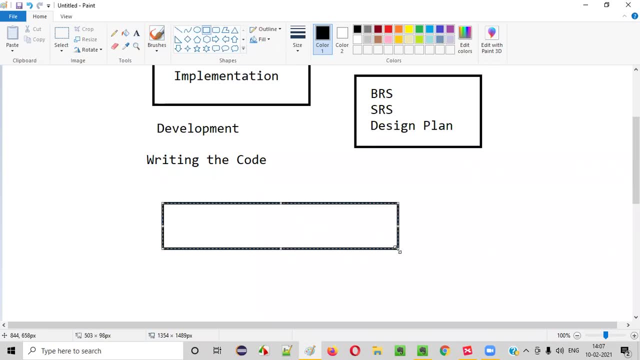 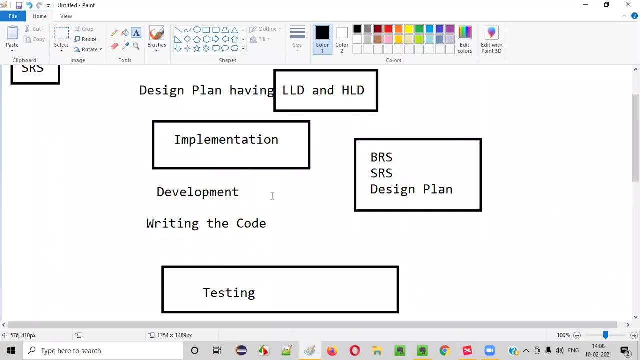 some XYZ functionalities or the complete functionality of the application, whatever it is. Then we'll move to the next phase. They will give that particular developed software for testing guys. The next phase is nothing but the testing phase. Once the development of this software- required software- is done, the development team will 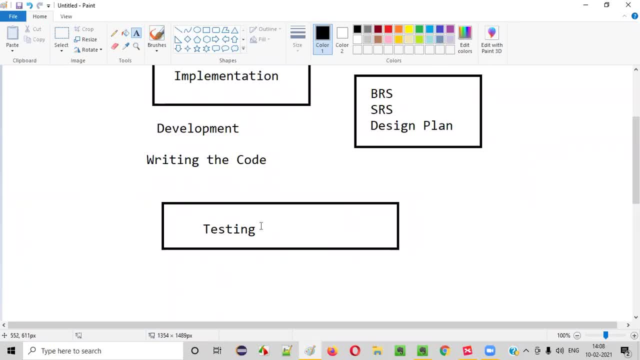 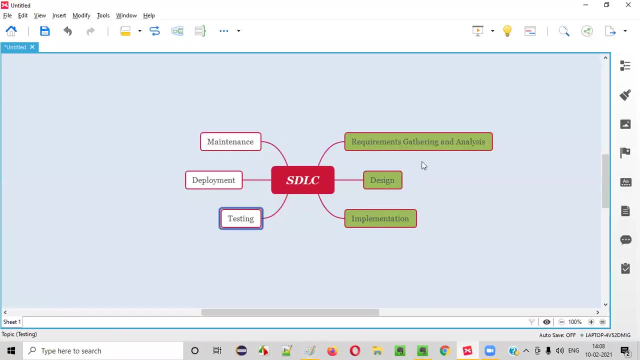 give the software for testing to the testing team. Here testing team will perform the testing. Till now, the first three phases guys, requirements gathering, analysis, design and implementation. The major focus was there with the developers only. Developers are more involved here in. 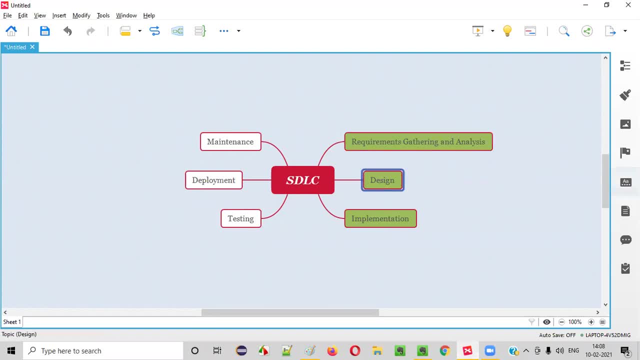 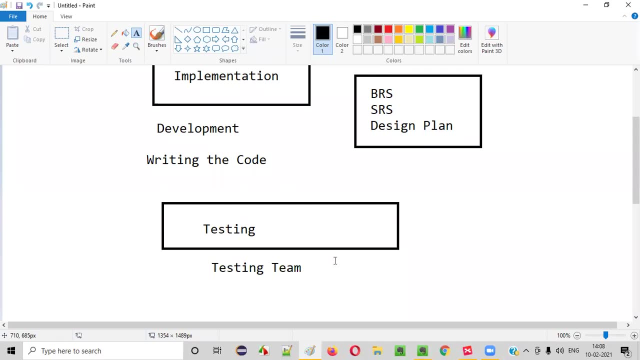 creation process. They created the SRS document, They created the design plan. They have written the code here. Now testing phase testing team will become more active guys. What they do is they will test this particular software, whatever the developed software given by the developers. 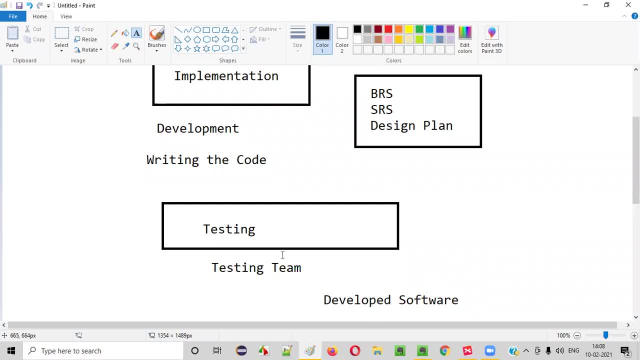 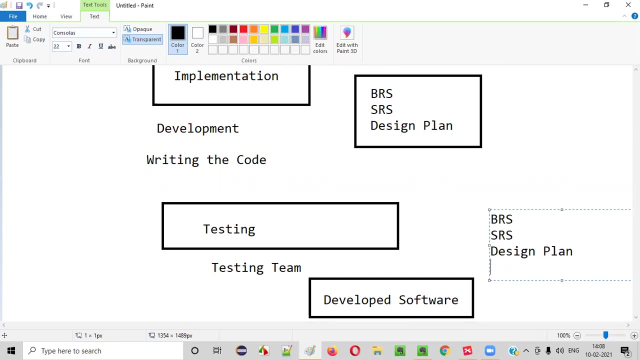 developed software. whatever the software that is developed and given to the testing team, Testing team will check whether this particular developed software, the software that is developed by the developers, is, according to this, BRS, SRS, design plans and any other docs that are either shared. 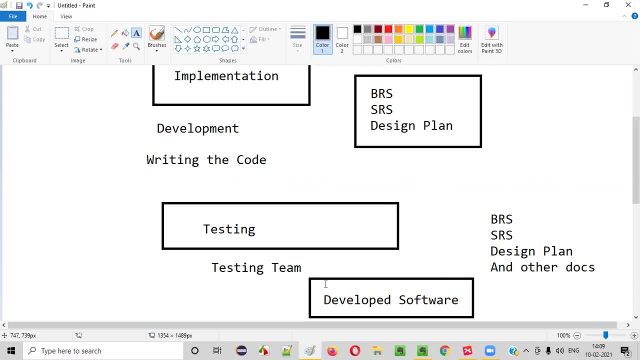 by the client or by the development team. They will use all this stuff to check whether this particular developed software is according to the previous documents or not. mainly the requirement documents requirements or not. That's the first thing that testing team will do. 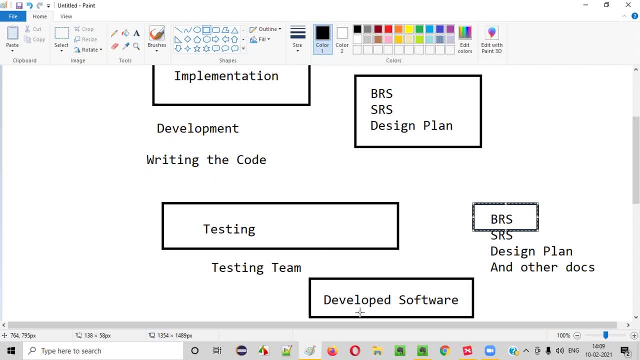 As part of testing. they will test the software. They will explore each and every application, each and every functionality of the software to see whether the software is built according to the requirements or not, mainly BRS. Also, they will check whether, whatever the software, that 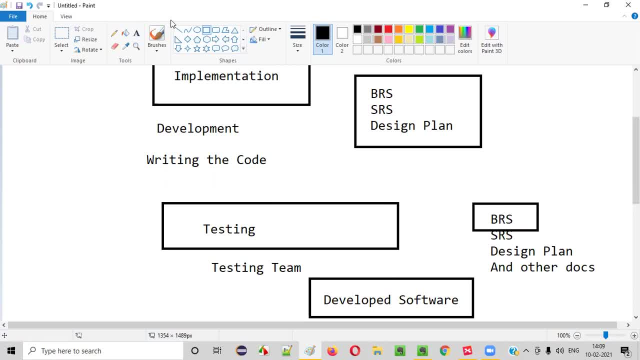 they have developed, even though it is according to the requirements, they also check whether this particular software is according to the user needs or not. So one thing is like this software should meet the business requirements. Another thing is whether, if it meets the business requirements but it doesn't meet the user needs, then software is 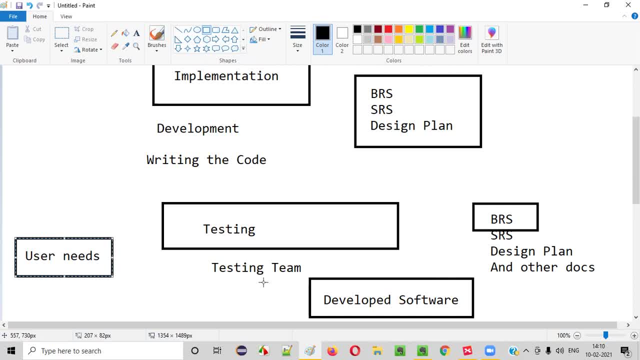 not helpful. So testing team will think in all directions. They will check whether this software is developed according to the requirements and also they will check whether- what about the user needs? whether the users will be able to properly use the software or not. Based on that, they will. 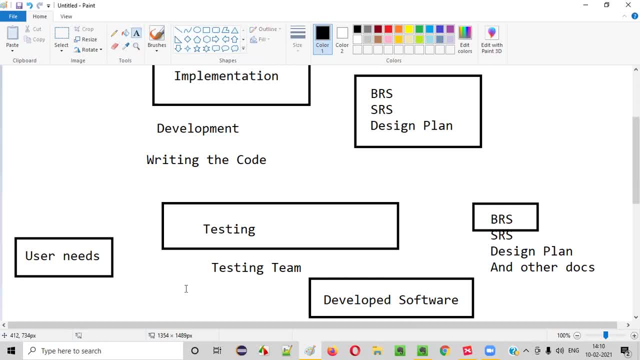 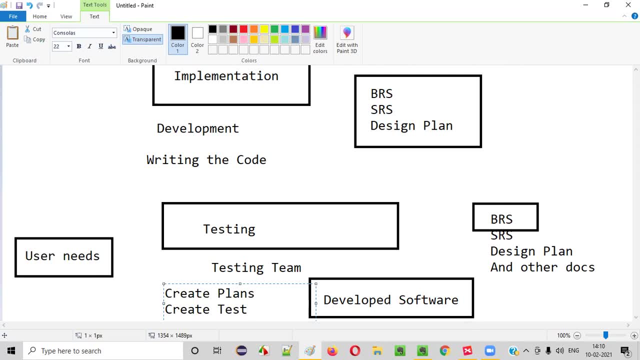 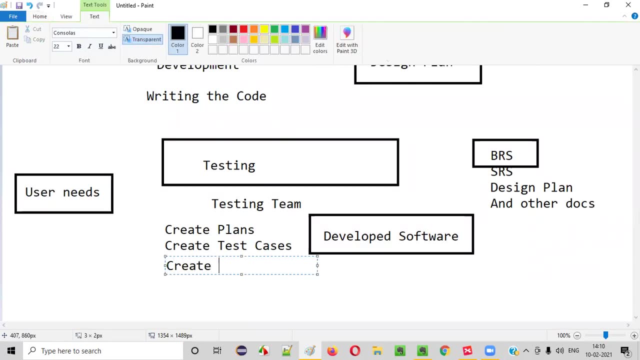 perform testing. So, as part of the testing testing team will create some test plans, test cases, a lot of stuff. Okay, I covered all this creation of plans, test cases, etc, etc. in the previous sessions. They will create some test reports. they will create. 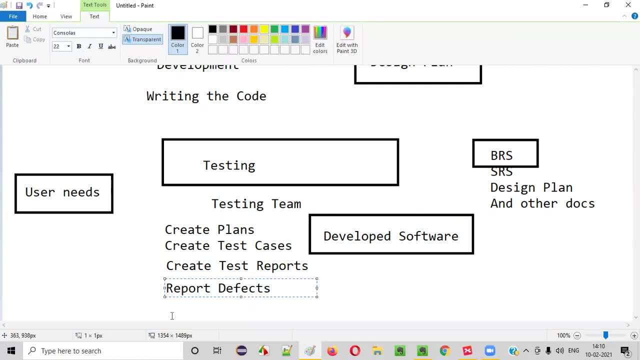 then they will report defects, they will close the defects. All the testing activities will be performed by the testing team in the testing case on this developed software to see whether the developed software is according to the requirements and all client requirements and user needs or not. 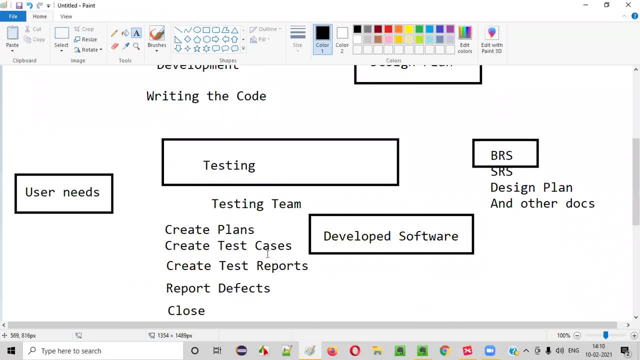 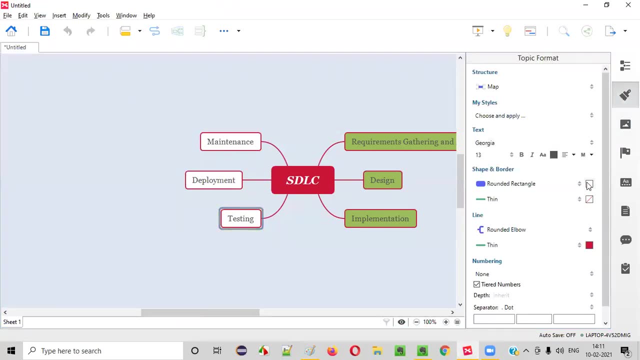 on that they will perform testing and so when, when developer, when testers find some defects, right, developers will fix it kind of thing will happen. that's fine. so this is a testing phase. testing phase is a phase in sdlc where the testing team perform the testing of the software to see if the 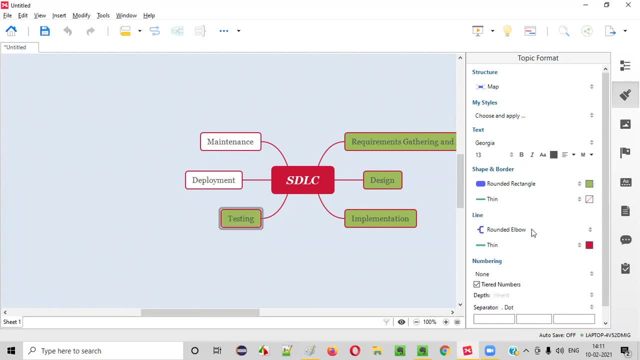 software is developed according to the requirements and user needs or not. and if it is not meeting any of those things, they will report the defects and they will do a lot other testing activities as part of this testing phase. now, after testing phase, guys, let's say here: developers have developed the 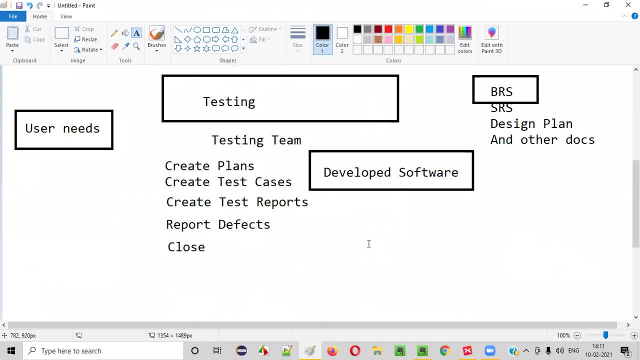 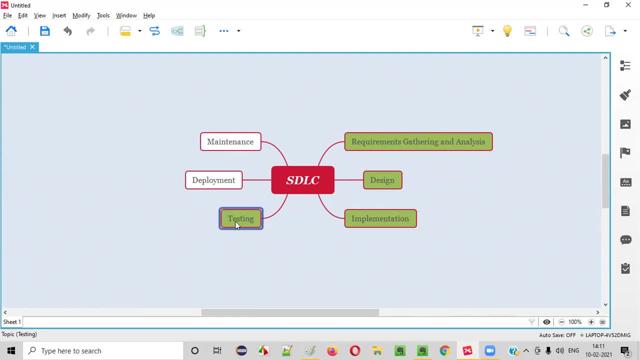 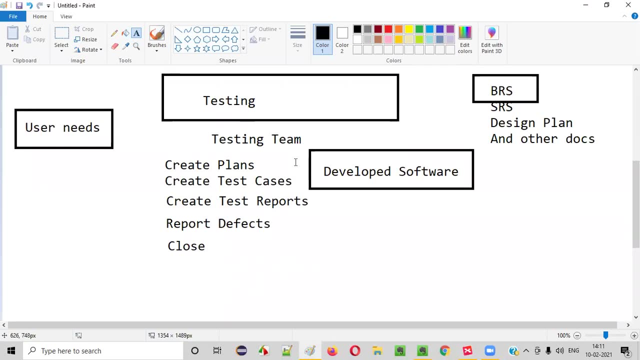 software testers have tested the software. okay, developers have completely developed the software in implementation phase. testers have completed testing the software in the testing phase and let's say the application is stable now. okay, let's say this application is stable now. what, uh, what will happen next, guys? the next phase is deployment phase. once the application is stable, guys, okay. 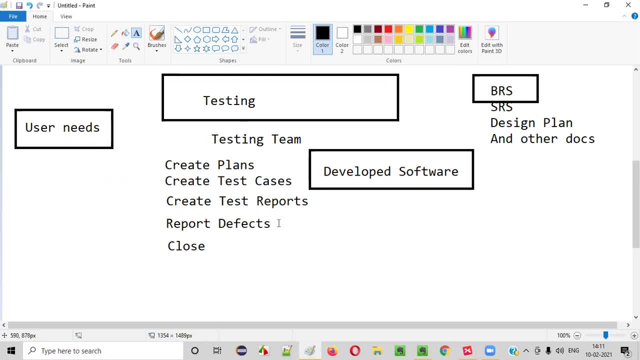 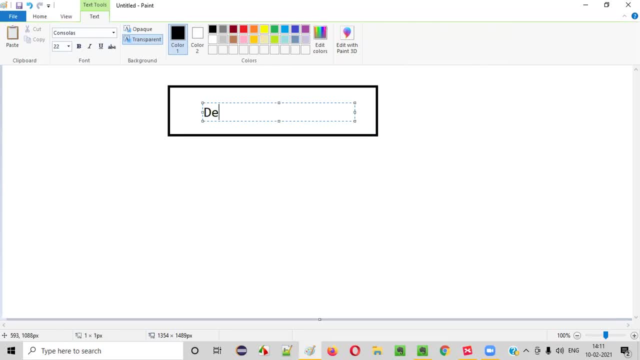 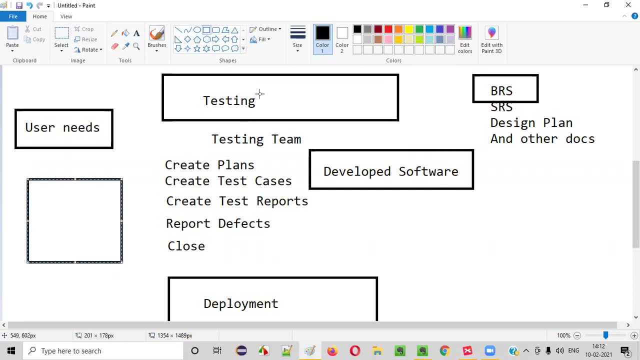 once this application is stable, properly, completely tested, then what happens is this software will be deployed into the production environment deployment phase. so here till now, guys testing team are using some environment. what is the environment that testing team will use for testing the software? we generally call that as staging environment. guys, i explained about staging environment in. 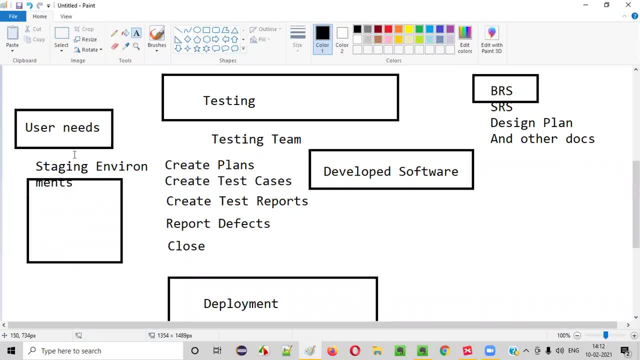 the previous sessions. okay, staging and in the staging environments, testing team will test that the application develop software. now, once the staging environment declares that, okay, once the testing team declares that this application developed software is stable and working fine in the staging environments, then then the day will come where this software need to be released. 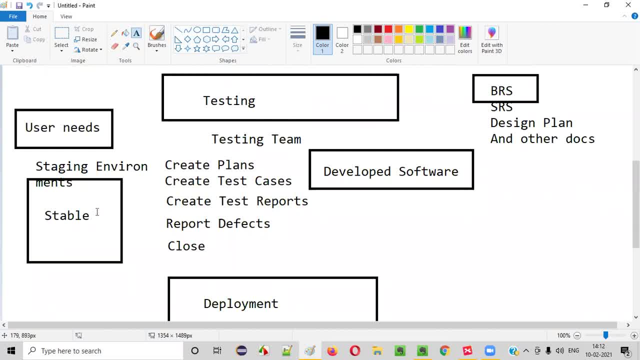 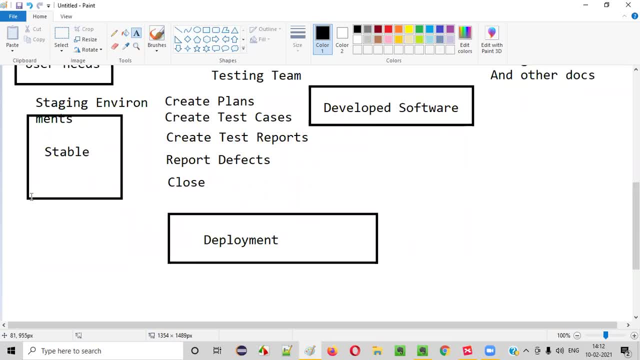 into the market right. a day will come where this particular software need to be released into the market. so how to do that? this code, okay, the developed software code- will be there in the staging environment now, right now. this code will be transferred to another environment as part of. 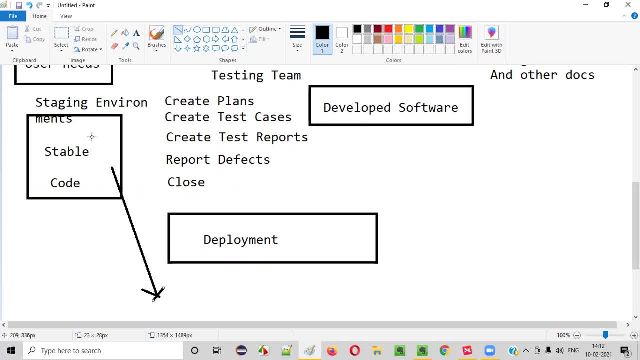 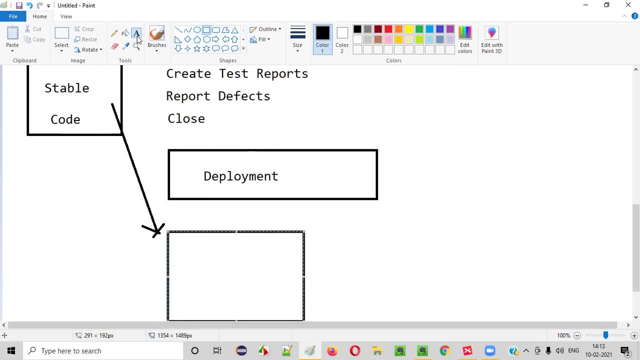 the deployment process, the working code, the stable working code, product product code will be transferred, deployed. you can say: okay, this stable code, uh, that, uh, that is certified by the testers, will be deployed by some other team. okay, we as testers, we are not going to deploy guys some. 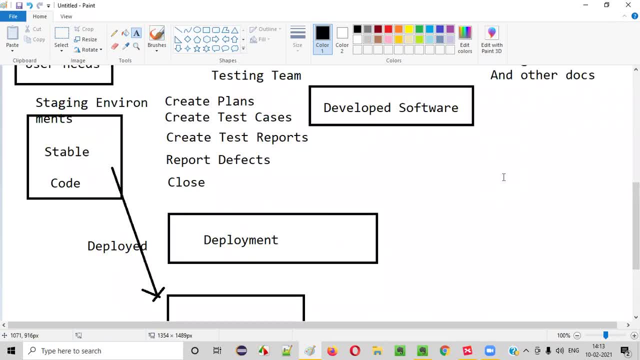 some xyz team will be there. okay, some other teams? some release engineering team. some different companies will have different teams for doing this. guys. okay, release engineering teams, kind of things. so operation teams: release engineering teams, such people. guys, what they will do is they will deploy this code, whatever the working code. 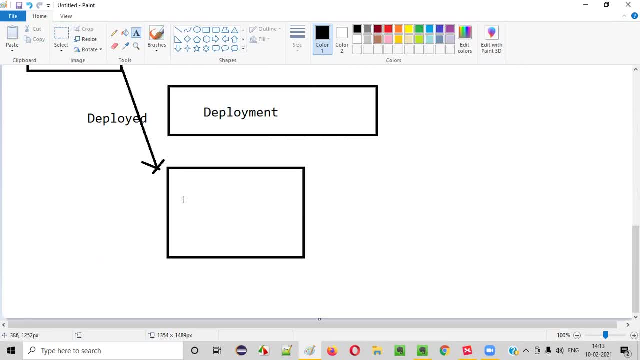 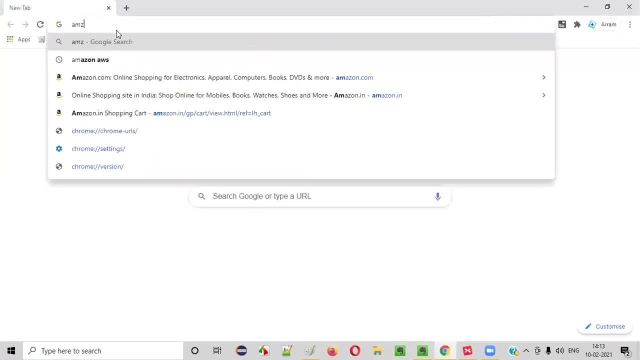 that testers have certified in the staging environments, that code they will deploy into the production environment. production environment is the live environment guys live environment, it's a live environment. for example, if i access this amazoncom, if i access this amazoncom, this amazoncom is currently in which environment guys production? 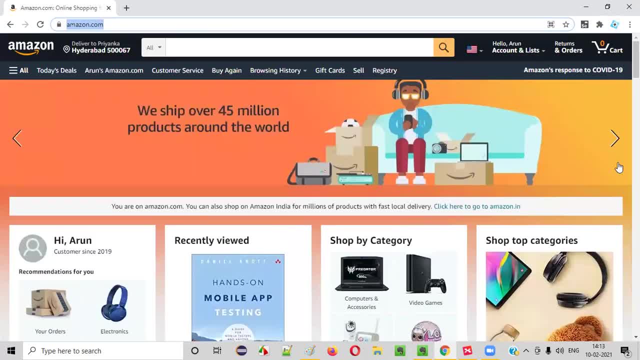 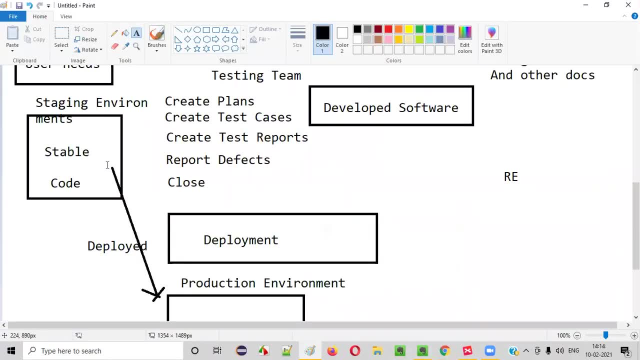 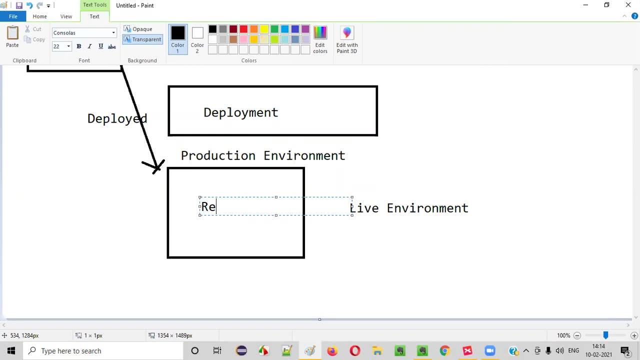 environment where every customer is using this software for purchasing some products online. right, so this is the production environment. guys like, once the code is good, only okay. once the code is good, only then only the code will be deployed into the production environment. that is, it is nothing but released into the market. the software is released into the market as part of 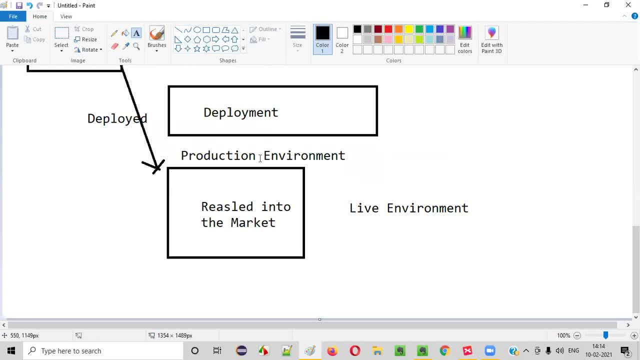 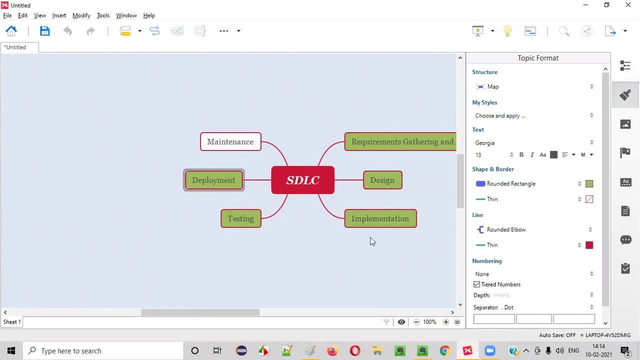 this deployment process, this deployment, uh okay, deployment phase is nothing but the phase in which the software is released into the market. the working code of the software is deployed into the production environment as part of releasing the software into the market. that is known as deployment phase, guys. 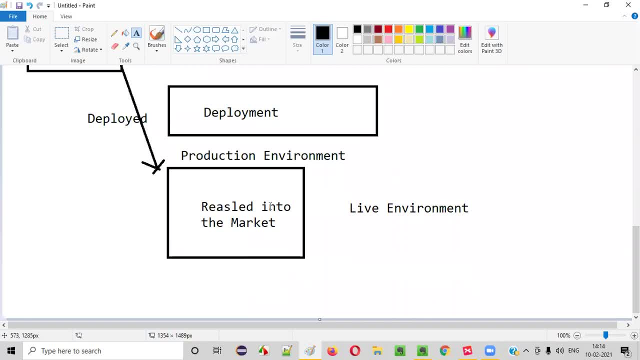 so. so if there are any issues in this production environment, what you will do, guys? let's say here in the production environment there are some defects observed by the customers, what will happen? happen. this is not a good sign right once the product is released into the market. defect should. 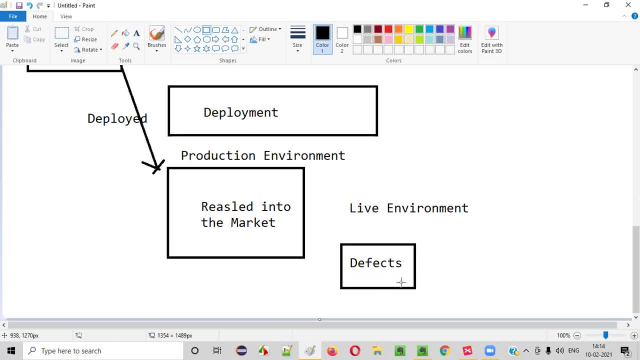 not come, guys. if it comes, then it is going to be serious, client will be unhappy and there will be a lot of- uh okay, scoldings, headaches and all a lot of stuff headache thing between the teams. okay, the client will come back to this xyz company who has developed this software and tested the software. 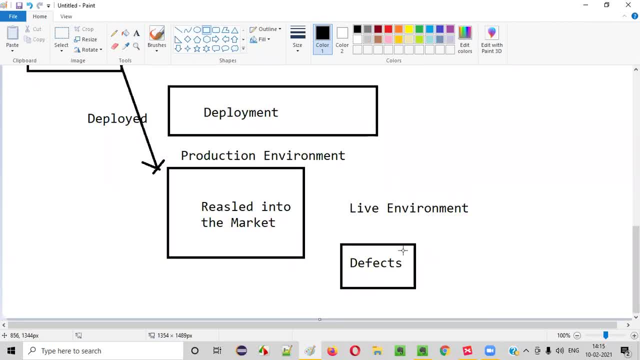 right, the client will be unhappy. that's kind of things will happen. but but sometimes, guys, some xyz defects will come anyhow and, uh, at this time, any problem is there. okay, so client will be unhappy and apart from that problem, guys, there is a solution also. that is, uh, something like production support, this xyz company, the developers of this developers. 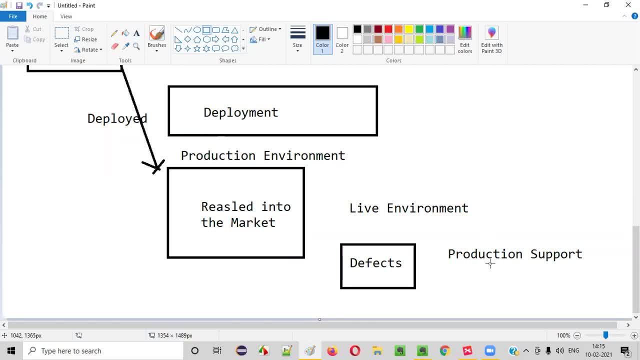 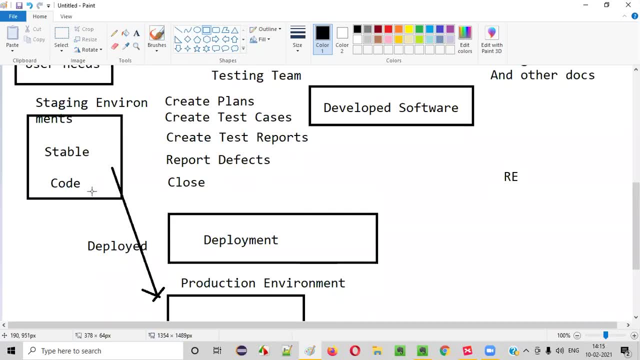 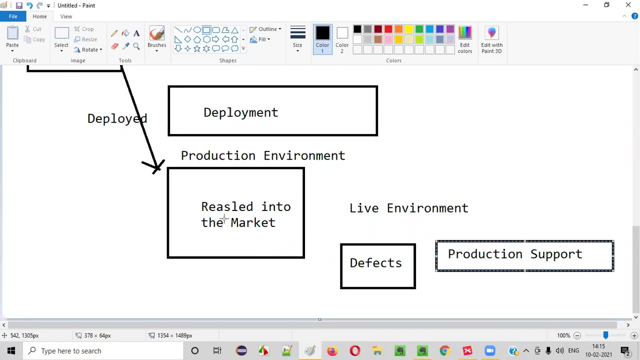 and testers of this xyz company will provide the production support. they will try to fix the defects in the production environment itself, which is not recommended. actually, generally defects are fixed in the staging environment, but but some situation came where they thought that the application is stable and they have released the application into the market. and after releasing into the 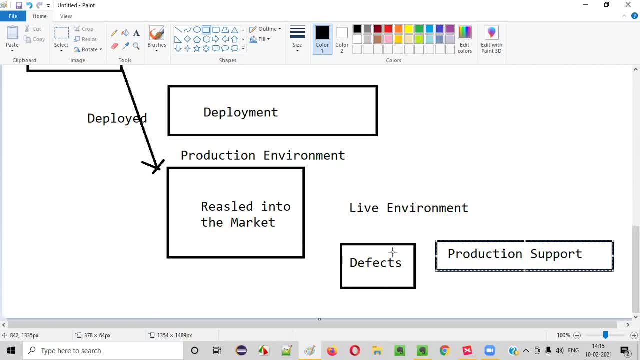 into the market. some customers- real-time customers of this application- have found the defects. there's a problem. it should not happen, guys. okay, the brand name and all those things will get affected for the client. so client will become definitely unhappy and xyz team is someone who will be. 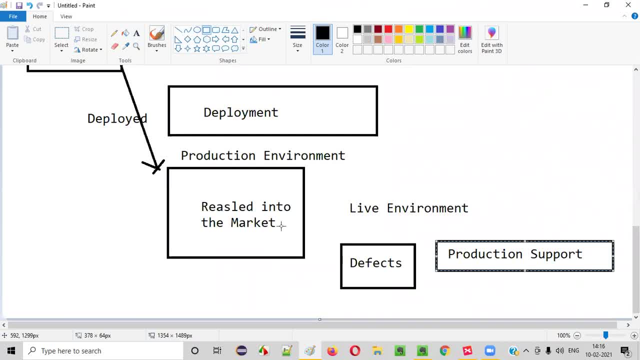 responsible for that, for delivering such kind of buggy application right? so their xyz company only has one solution, that is, they have to provide the production support. that means they have to give the developers and testers to fix. okay, they have to use the developers and testers to fix. 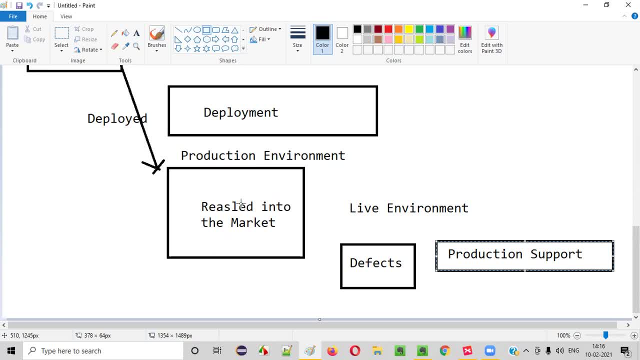 this particular defects while the production environment is live, which is very risky, guys. okay, this production support is very risky. when they fix something, it may cause some other side effects, right, so such kind of experiments we should not be doing in the production environment. but if there is no other way, they use the production support to fix such kind of issues. 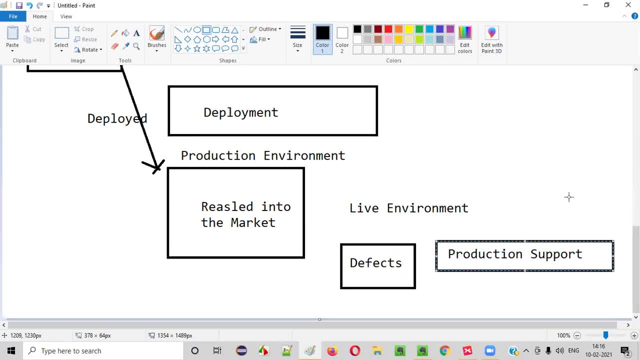 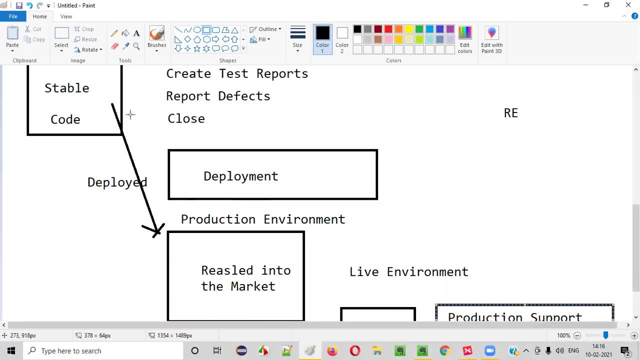 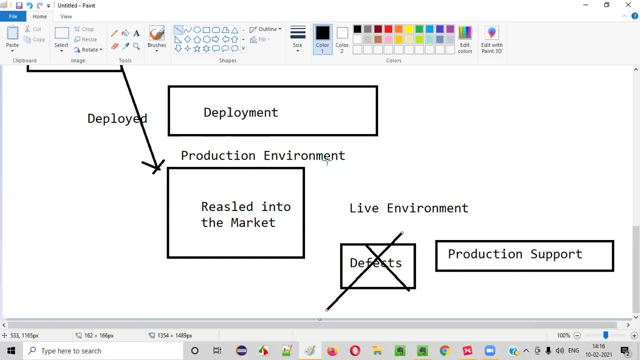 and there are no defects. also, once the application is like okay, once the production environment is live, then released into the market, software is linked to the market, then let's say there are no defects, came and things are going fine. so that is this. the end is the deployment phase, the final. 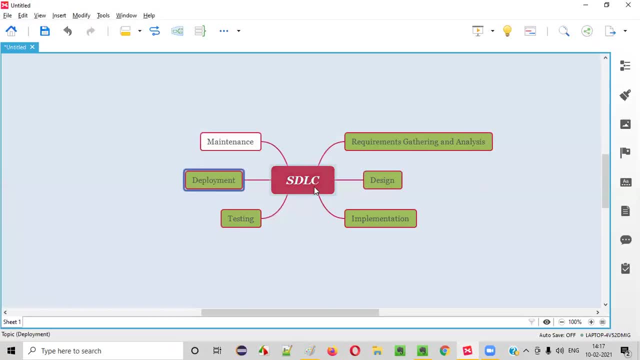 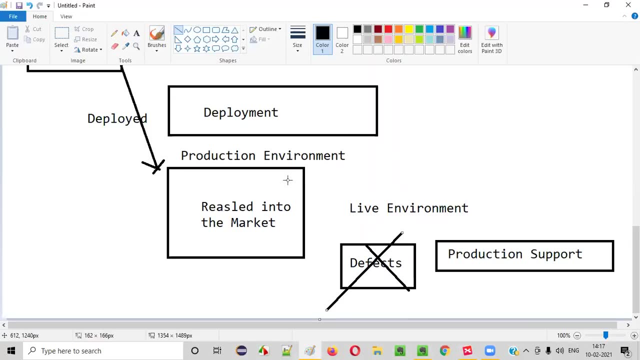 phase. no, guys, there is one more phase in the sdlc. there is one more phase, that is, maintenance phase. when does it come into picture? let's say tomorrow, while the application, while the production environment, things are going fine, okay, application is live and properly released into the market without any bugs, and all tomorrow. 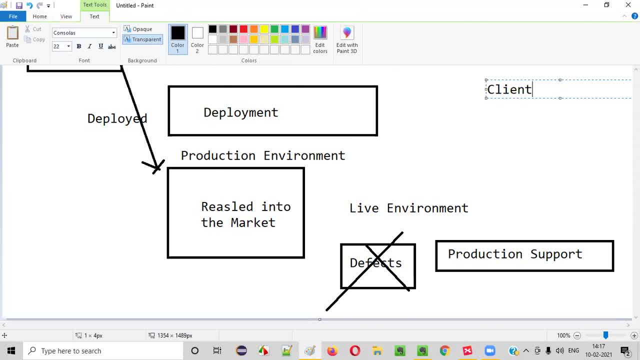 guys, client may get another requirement. okay, customers, uh, you see, a lot of competition is there in the market, right? so when you create a website, another person also will create the same website. such kind of competition is there in the market. so what client will do is, uh, client. 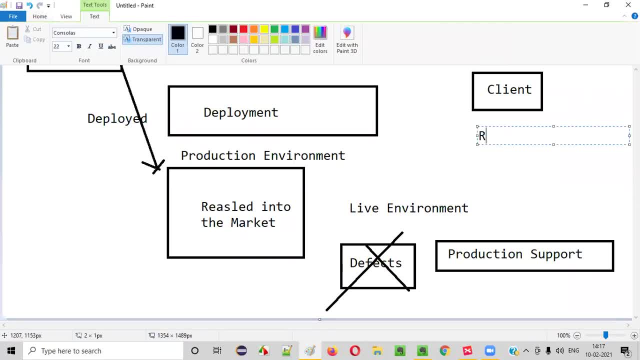 will keep on, uh, like, uh, keep on getting some requirements, guys, some new requirements, you may get some new requirements. okay, he will get to know about some new ideas from the customers, or new requirements from the customers, or, and uh, you know to be to be good in the market, uh, we need to implement some some more. 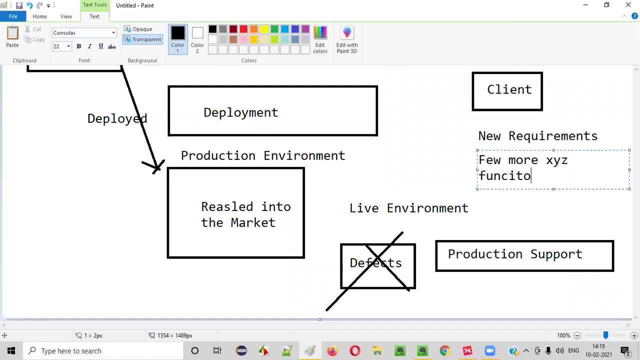 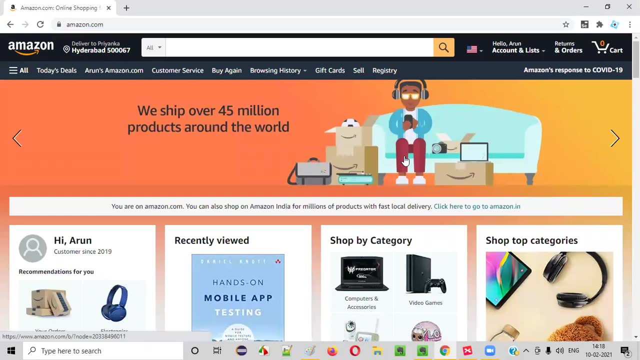 few more, few more xyz functionalities like that. so this applications keep on changing right. for example, today amazoncom is there, okay, so amazoncom may look something like this today, but tomorrow, guys, uh, based on the need, okay, based on the need of the customers who are purchasing the products from. 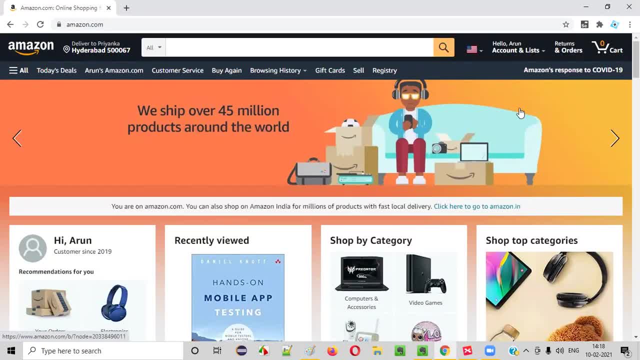 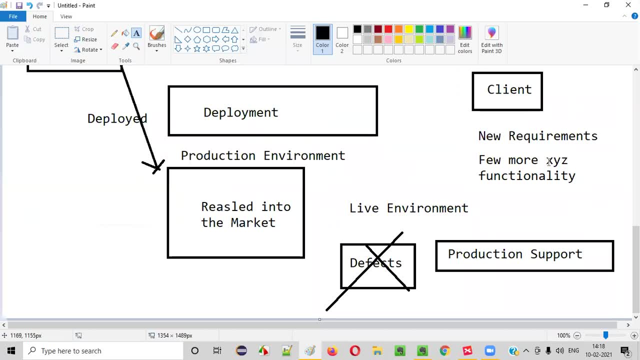 this amazon. new options will keep on coming, guys right, because of the market changes and all some new functionalities this amazoncom people have to implement. those are the nothing but the new requirements. sometimes existing functionalities need to be updated. okay, some, uh sometimes some existing functionalities need to be removed which are outdated. a lot of things may happen, guys that. 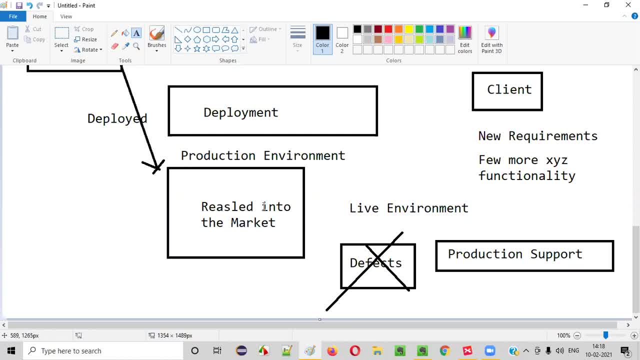 where you will do all those changes to the application, guys, once the product is released into the market, then where you will. where you will do all these things: how to get this new requirement, new functionalities added to the existing application, how to update the existing functionalities, how to remove the outdated functionalities. all those things will happen as. 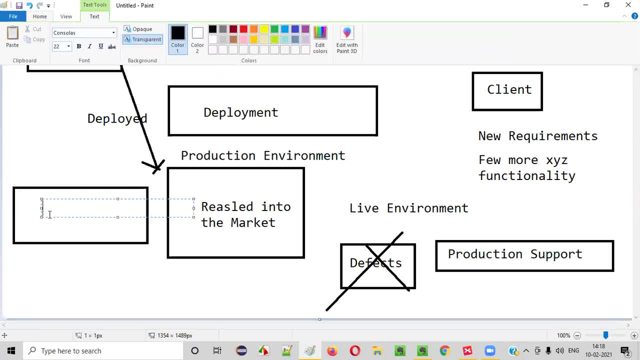 part of the last phase of sdlc, guys, that is maintenance phase. okay, in the maintenance phase, any new requirements of new functionalities that are need to be added to the existing application will be here. developers will will do that. yes, again the same thing. developers, testers will be there, testers will be testing it. 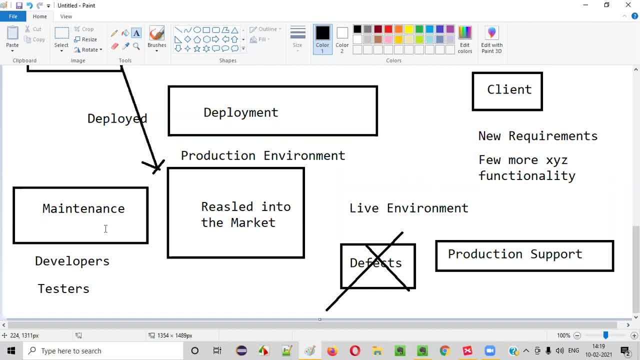 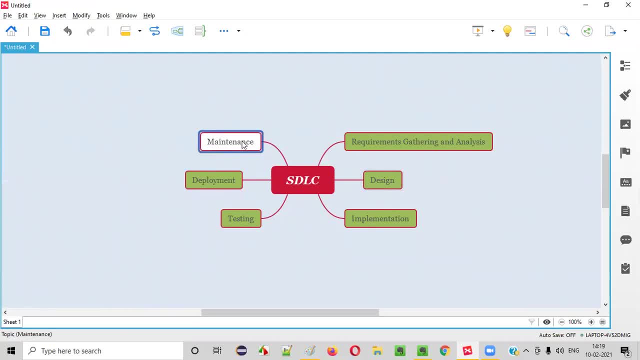 to see whether the new functionality is added or properly added or not. this phase is known as maintaining phase. once the application is released into the market, then it will go to the maintenance phase where development team and testing team will help the client in adding more new features. 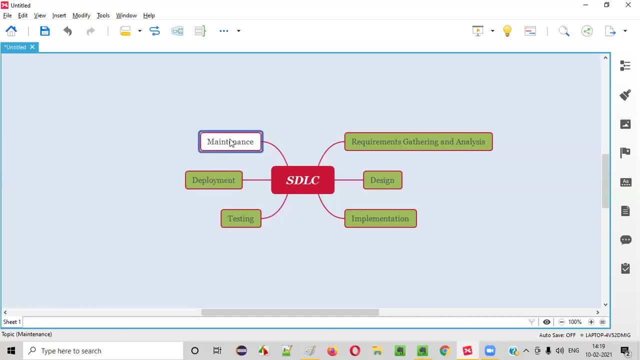 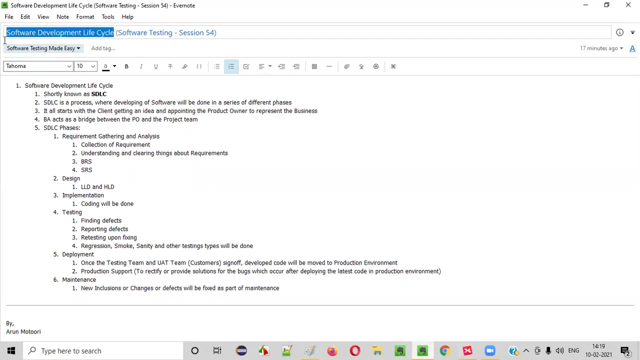 or updating the existing features or testing the features or whatever it is okay, fixing the defects, fixing the past defects or whatever it is okay. that will happen in the maintenance phase. so that final phase is nothing but the maintenance phase. so hope, guys, you understood sdlc in a detailed. 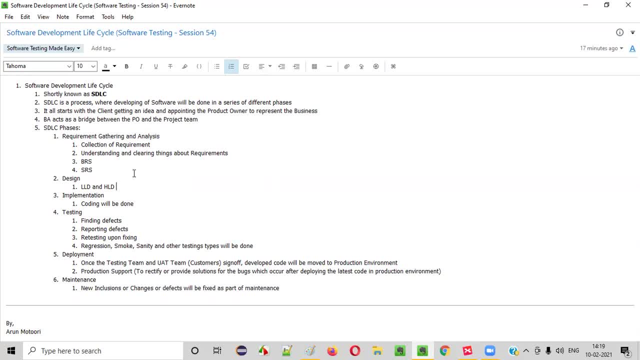 manner in this session. okay, these are the several phases of sdlc, guys, that is, the requirements gathering and analysis phase, design phase, implementation phase, testing phase, deployment phase and maintenance phase. so that's it, guys. thank you bye.